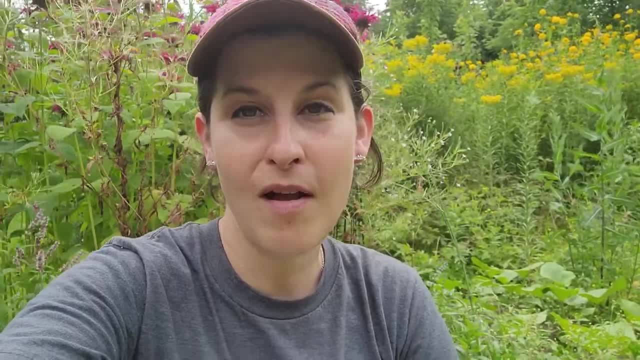 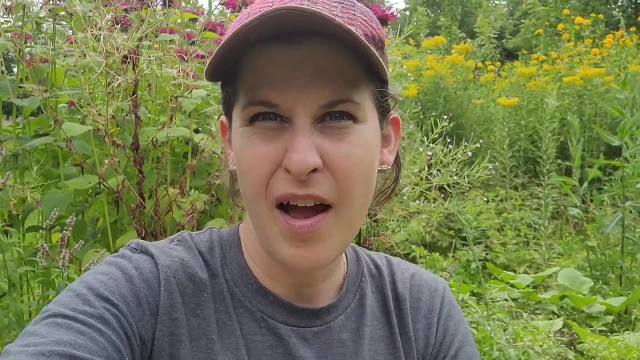 natural botanicals in them as well, as we'll do some other fun soaps as well. It's glycerin soap, so it's for folks that really want to make soap quickly, that don't want to be messing around with lye- you know some of those chemicals that can cause caustic burns when you're making the soap. 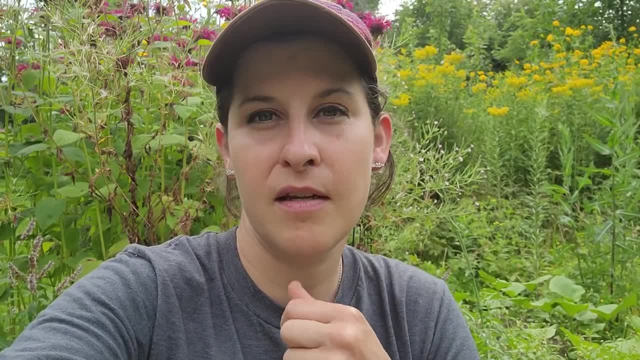 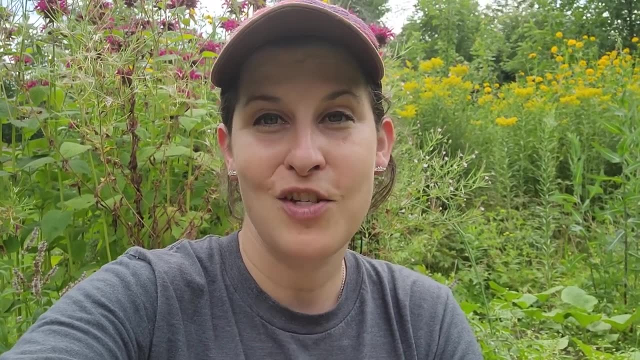 making process and they want to try something that's really good for the skin. Glycerin is a humectant, so it keeps that moisture in your skin, and sort of hypoallergenic too. So let's check out what we're going to do today in the kitchen. So earlier this week I harvested some flower petals. 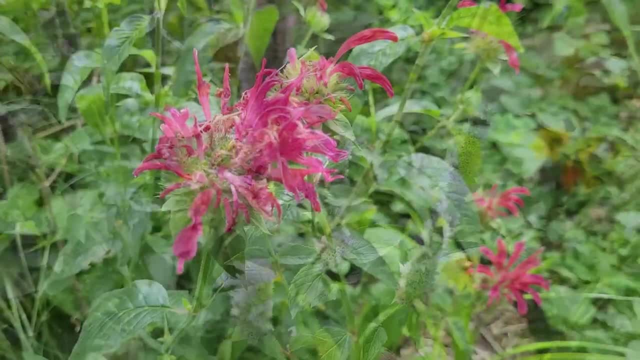 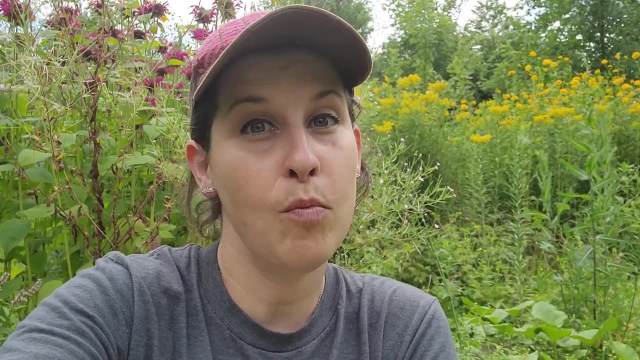 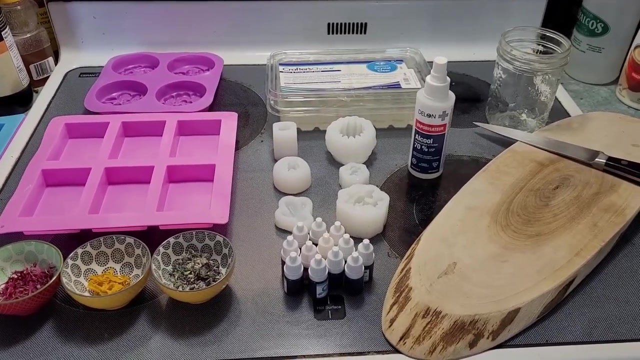 and I dehydrated them for today's soap making recipe. So let's head on into the kitchen and get making some soap. This soap recipe is really quick and easy and you'll have soap within two hours, Let's go. So here we are, set up in the kitchen and I've got everything that we need to make the 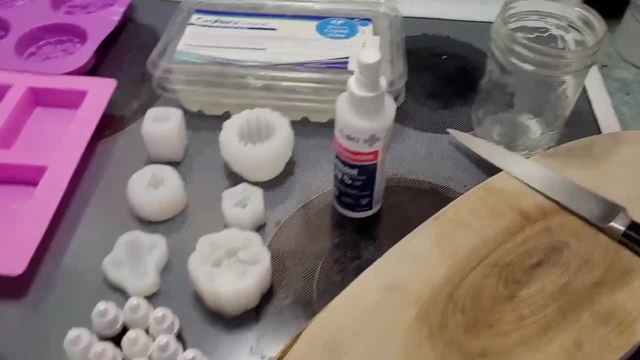 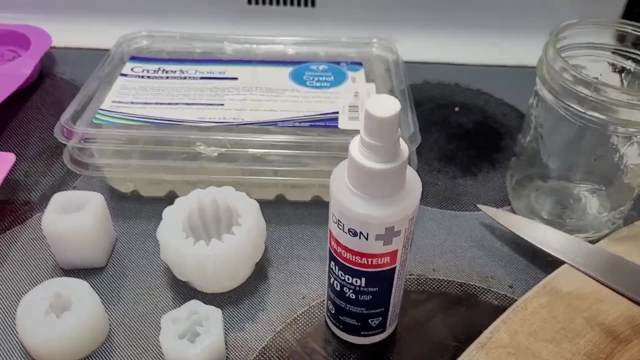 glycerin soap. So let's take a look. We'll need a cutting board, a little jar to mix the glycerin in some rubbing alcohol, because glycerin soap tends to get little bubbles in it. We want to help prevent that. I picked up some crafter's choice premium crystal clear glycerin, handmade. 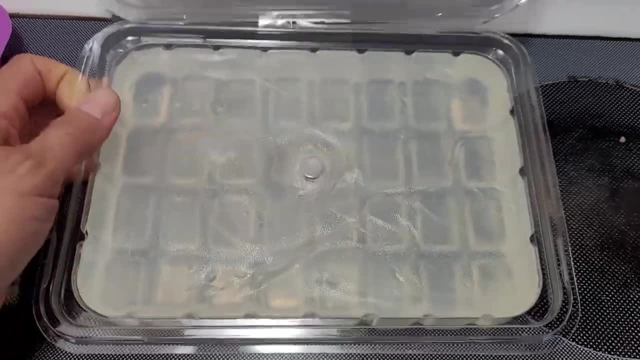 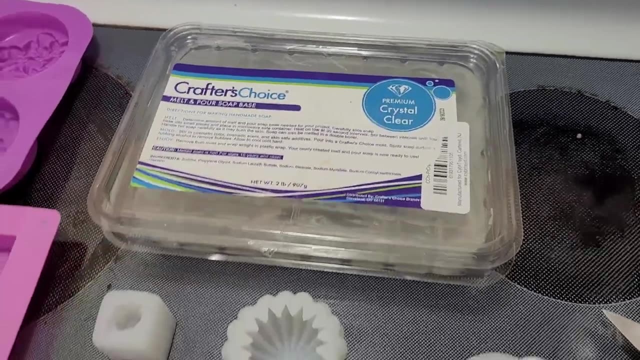 soap base So we can see how clear that is. You can see my hands through there. You know you can pick up stuff like this off Amazon- That's where I got this one- or, you know, Hobby Lobby or Michaels, So it's super easy. And then, of course, your molds. Now I've got some fancy molds here. They're. 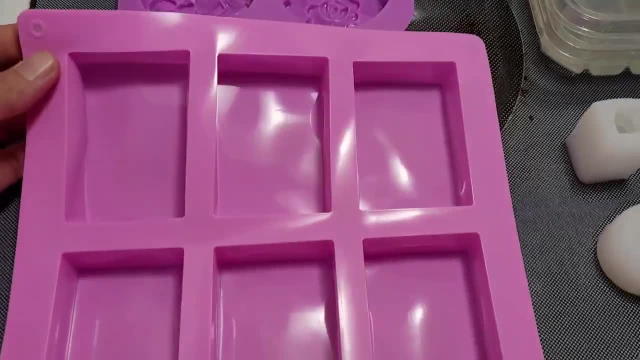 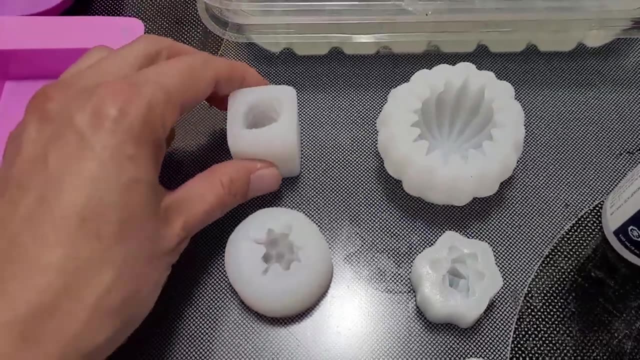 all silicone. This one's got some flower patterns in it. This one's just your standard soap bars. I'm going to try a little experiment today with one or more of these. These are actually molds for succulent cacti, So I thought that would be pretty cute for like little mini soaps, You know. that's a great idea. I'm going to try this out. I'm going to put it in the fridge. I'm going to put it in the fridge. You know, I'm going to put it in the fridge, So it's just going to be okay. 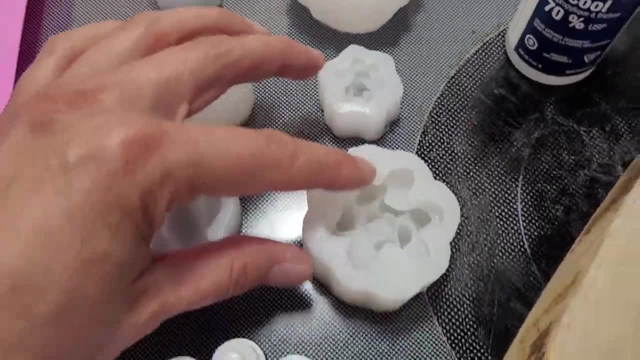 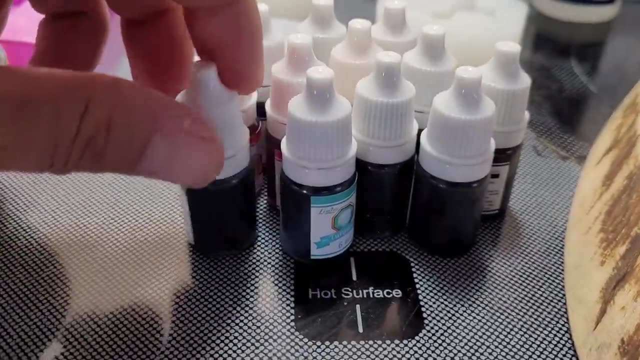 soaps. you know we have guests and stuff like that, so I'm going to experiment with those. those are new off Amazon and, of course, down here. I've got sort of my food grade food coloring. I use any like make sure the food coloring is safe for like food or for cosmetics. so I've got different colors. 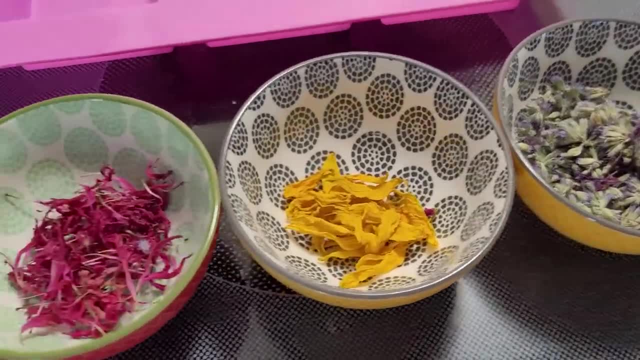 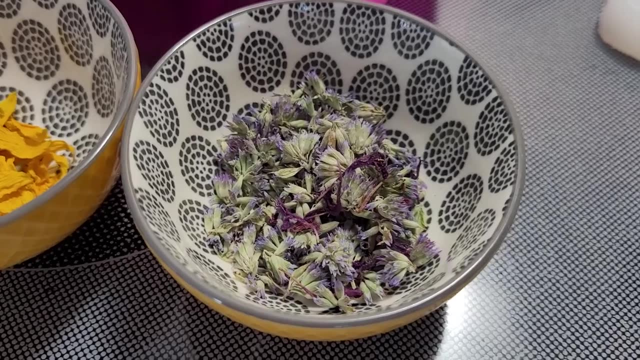 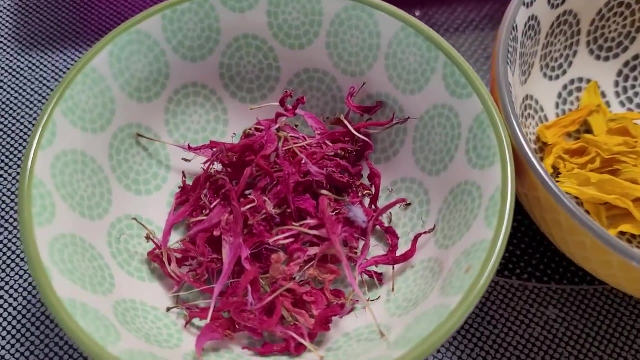 here we can mix, and then from the garden I've dried some petals from some of my flowers, so this one is star anise, that one smells like licorice, and this one right here, this is from some black-eyed Susans, and this one is my wild bee. well, not my wild bee bomb, this is just like a. 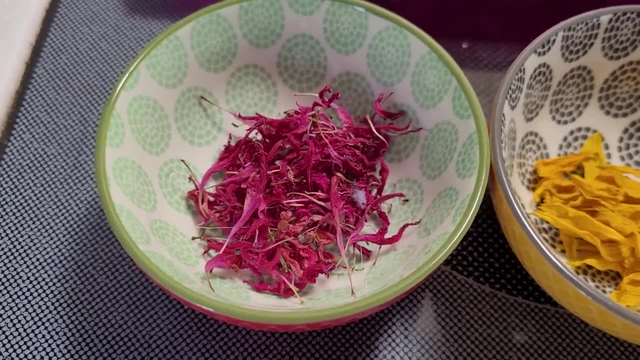 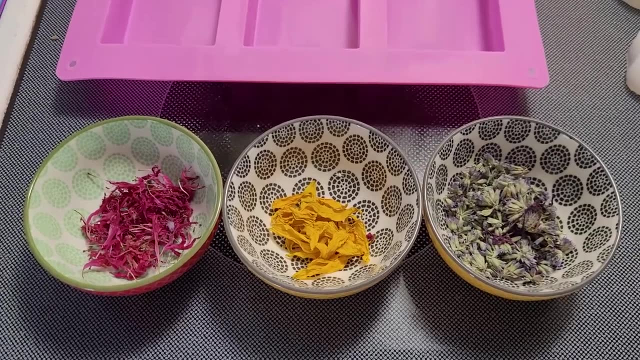 bee bomb that it's kind of like a pinkish color. the wild bee bomb slash bergamot is a beautiful purple color, so we'll put these in some of the soap bars as well. so let's get started. so the first thing we're going to want to do is guesstimate how much glycerin we need for our project. I might 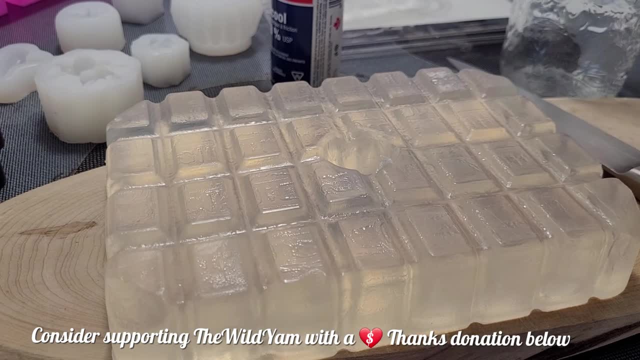 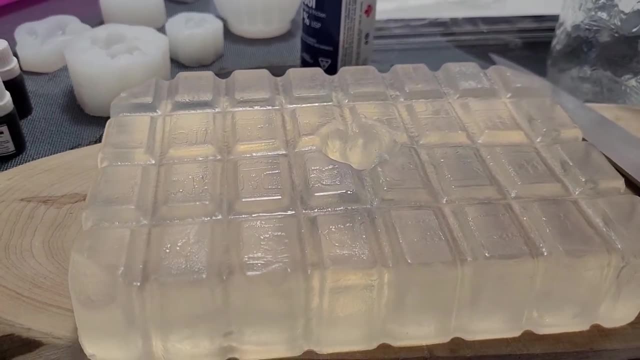 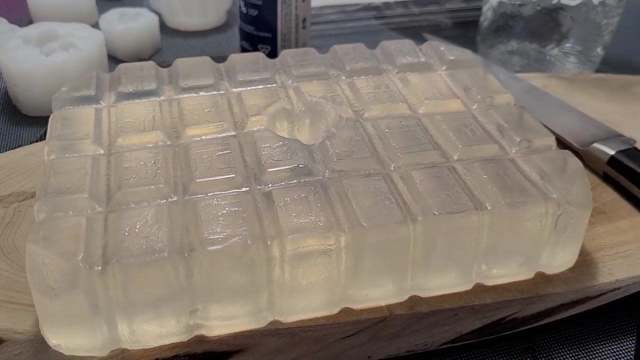 do this in a few stages. I might start with, you know, pouring out the little flower ones first. do my different like color dyes and things like that. it will kind of harden over time so I might want to work rather quickly. so let's do the flower ones first. I'll take off a few chunks of this and we'll 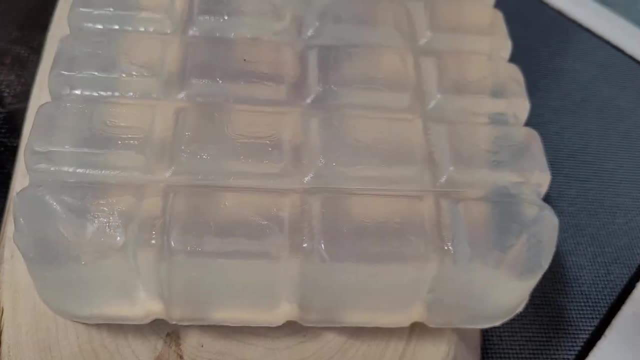 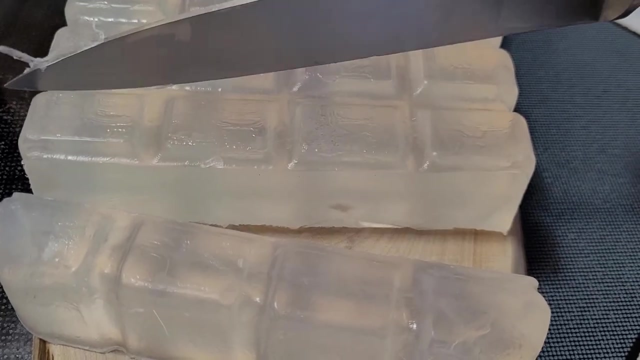 get it set up in the microwave. it's typically not very difficult to cut. you can kind of cut it down these little score marks. here it's. you can see it's just like butter kind of going through here, like kind of like firm texture of butter. I'm going to kind of cut these into the little cubes. 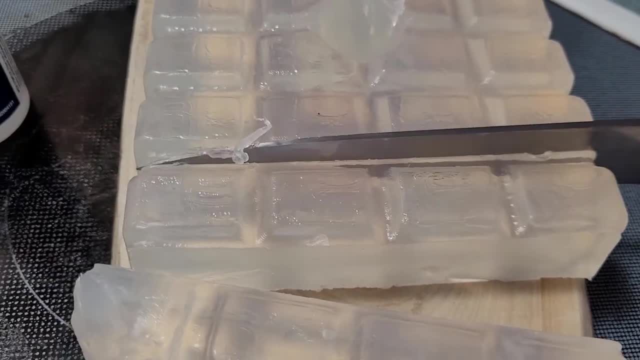 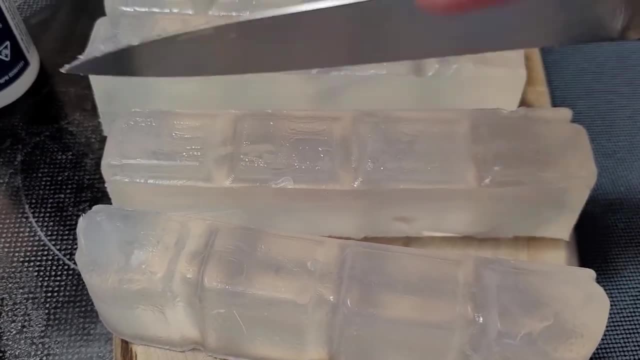 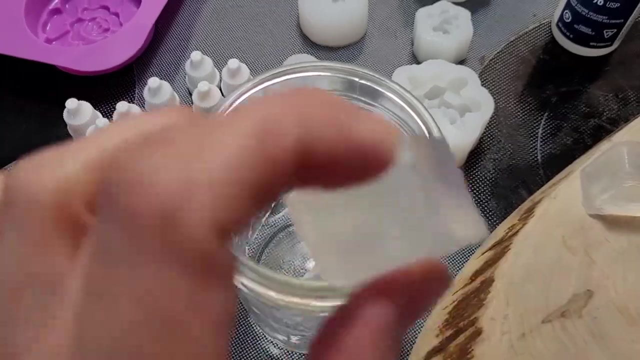 that they have them pre cut out at, just so it melts a lot easier. I kind of guess how much I'm going to need for this little project. maybe, I don't know. this is probably too much, but let's go with this to start. all right, I've got this glass jar here and I'm just going to put a few little chunks. 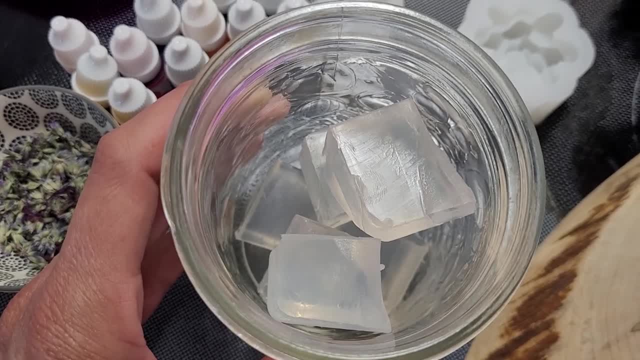 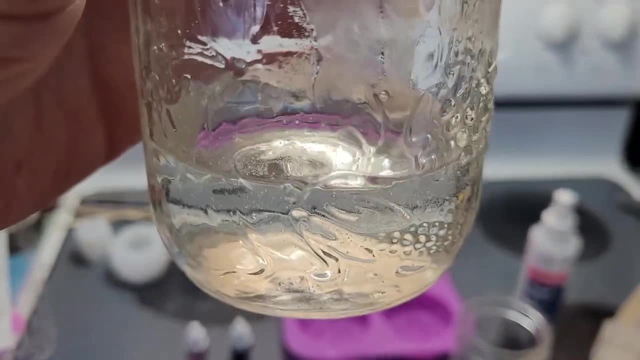 in there. all right, let's start melting this. we're going to go at 30 second intervals in the microwave until it's completely melted, and remember this will be extremely hot, so be very careful. all right, so this is 30 seconds in and it's looking great. so this is the point. if you wanted to add essential oils or anything like that, you 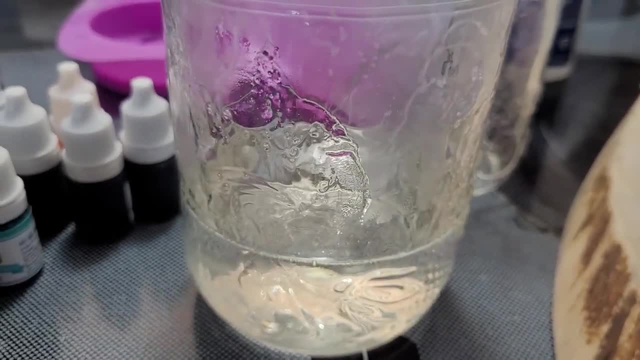 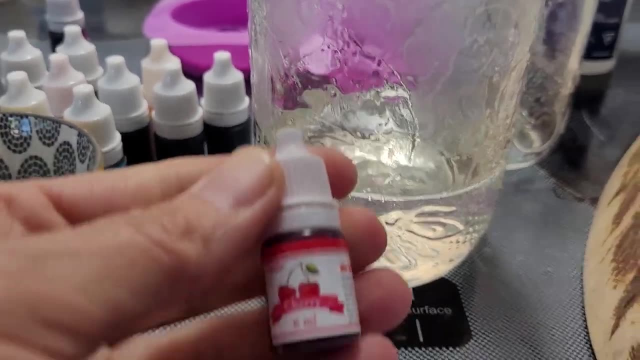 can add that in. right now I'm going to start pouring this into the molds. if you want it clear, you leave like that. I want to do this one with a little bit of red, so we're going to go in with a little bit of the cherry. remember, less is more with this, or you're gonna have an extremely intense. 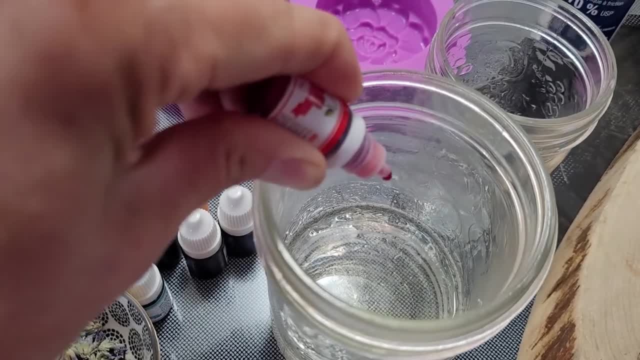 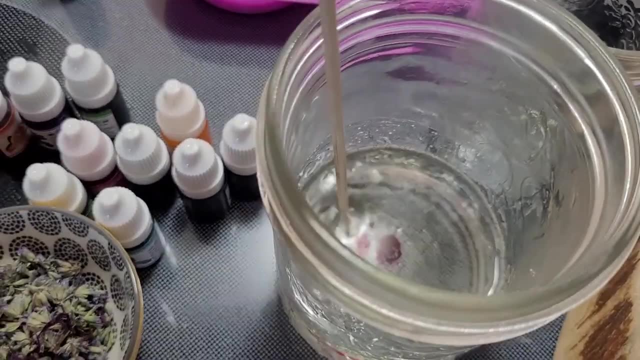 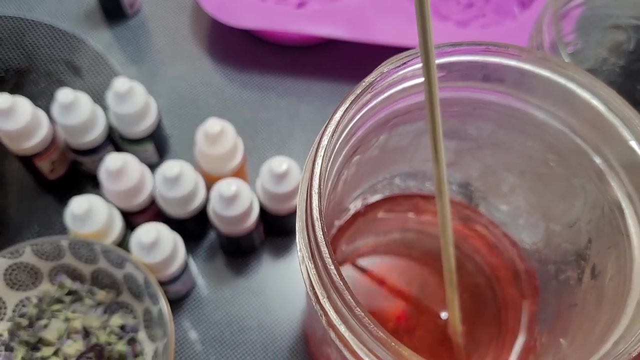 color. put a couple little drops in here, hope they don't overdo it, or you can always reassess if you need. there's three drops. I've got a little stir stick here. I'm going to go ahead and put that in here. I'm going to kind of go in and, yeah, see three drops. look how red. that is a little bit more. 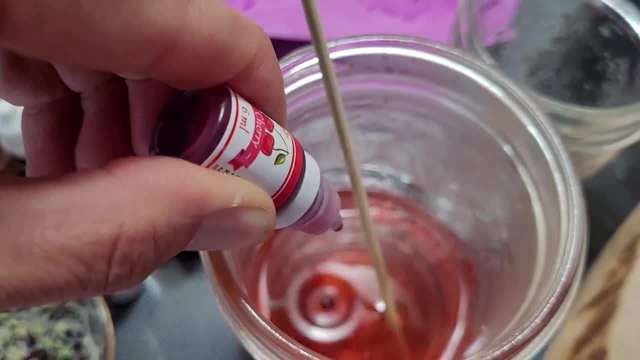 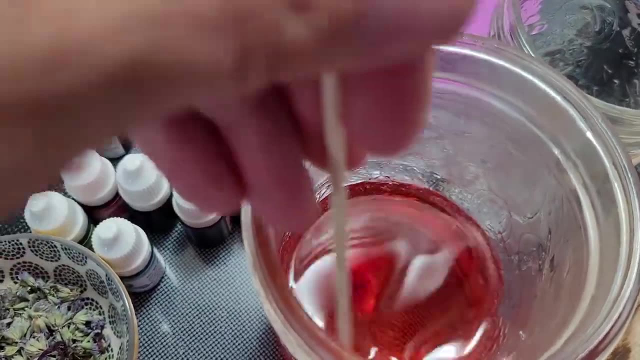 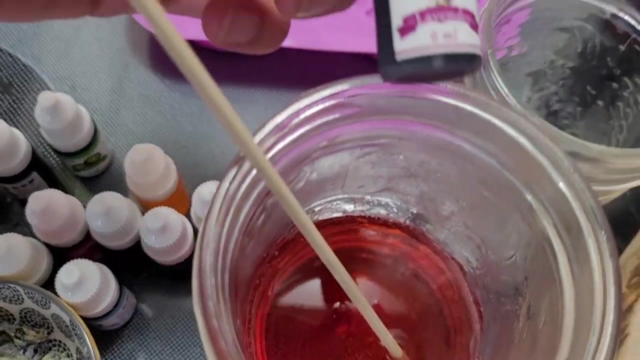 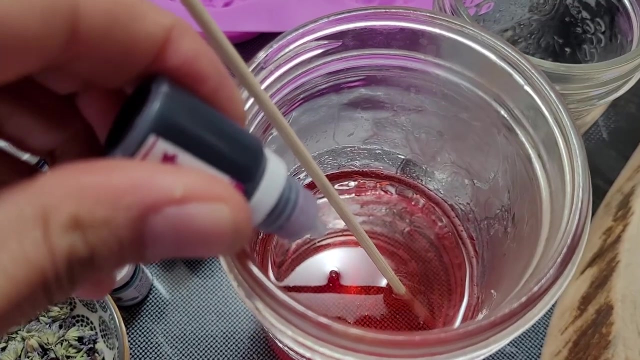 there too, maybe. oh geez, I was three whoops. that looks cute. no, should experiment with more colors. let's see what I got. I have like a lavender here. we could add a mix of that. I don't know my color. know what we can expect. little charts online you guys can get and figure it out. let's do a couple. 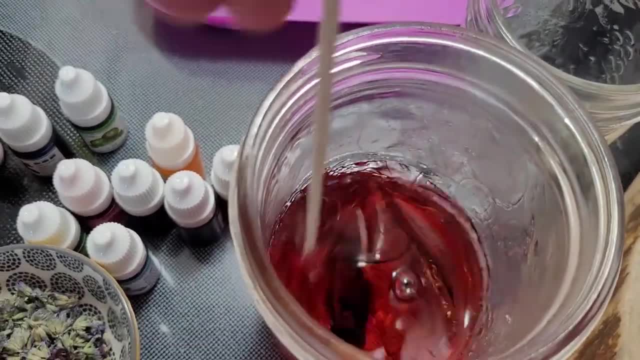 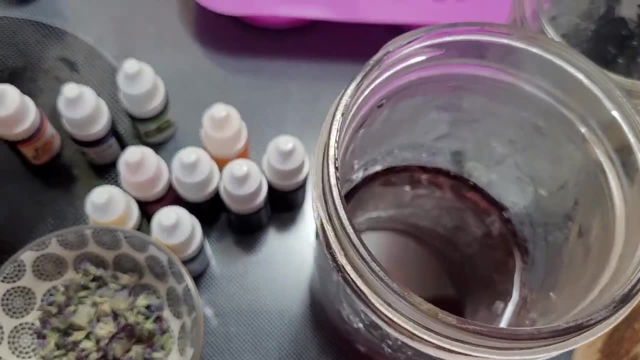 wow, geez, I need to do that. all right, I think that'll be pretty good. oh, it's kind of a nice dark wine color. all right, let's get this poured here. all right, so we're going to start in this one. remember, this is like super hot, I'm just going to pour it in this. one's just like the rose mold. 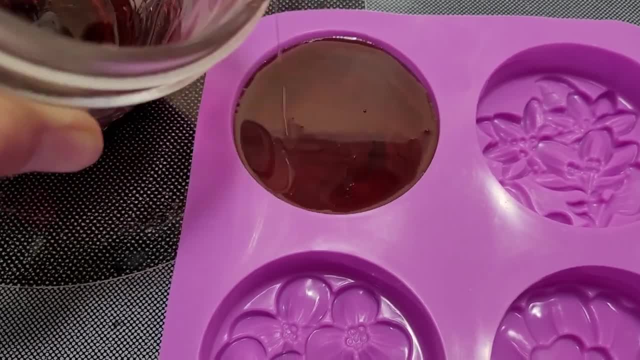 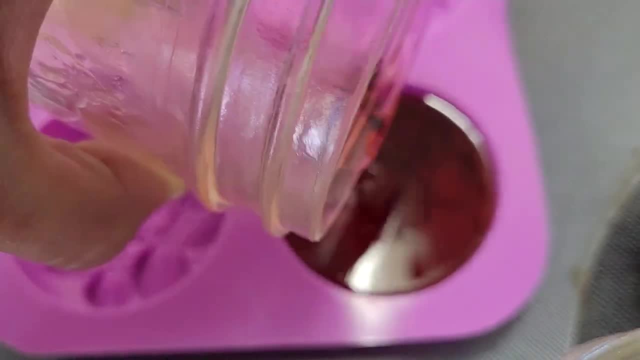 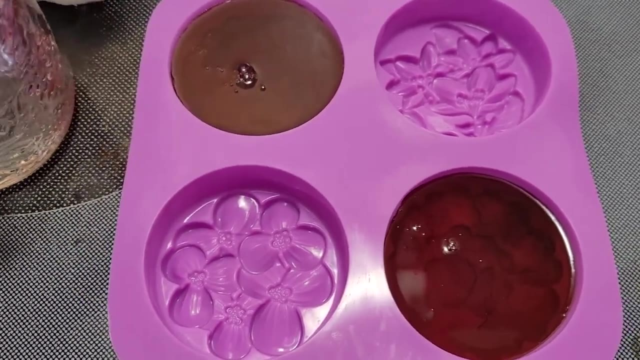 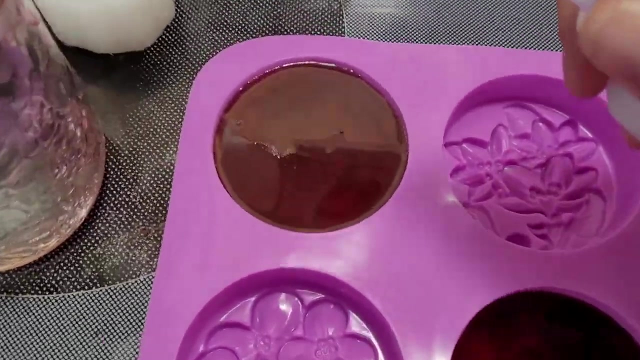 oh, that's cool, and then I'm going to do this one as well, suit this red one as well, and that should be it. okay, perfect now, because glycerin soap is prone to developing these little air bubbles you can see on the surface there. what I like to do is go with the alcohol and just spread. oh see, it's gone, you do. 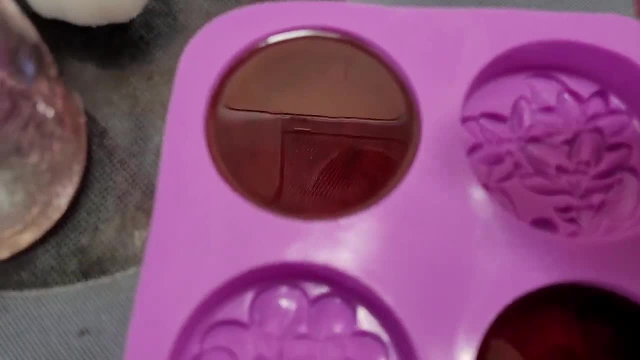 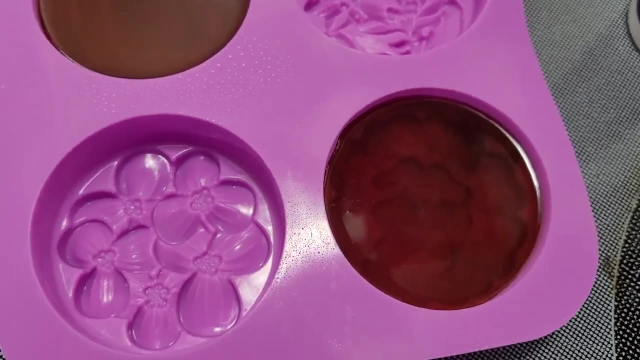 that see the bubbles gone. some people with this at the bottom as well, because you can get bubbles at the bottom of your soap molds- soap mold, so okay, so there's that one. so I'm just going to clean out my little jar and I'm going to 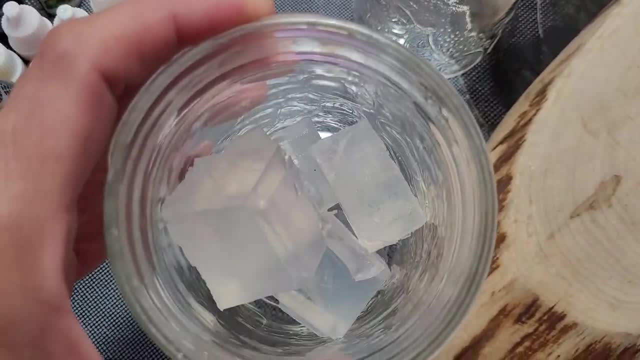 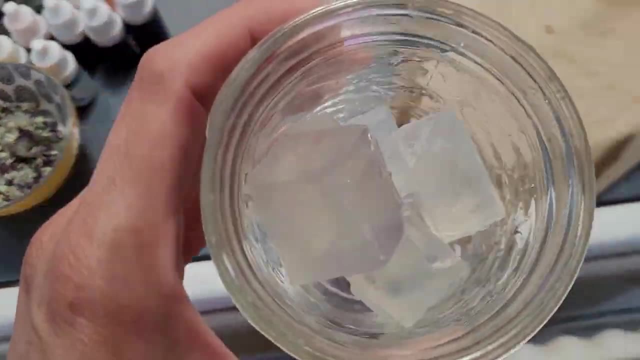 do these guys next. different color, okay, so all cleaned out again. it's soap, so just washes out pretty fast. so about six of these. it seems like each of these takes about three of the cubes, so we're going to do that right now. all right, so we're all set. I'm going to try something a bit. 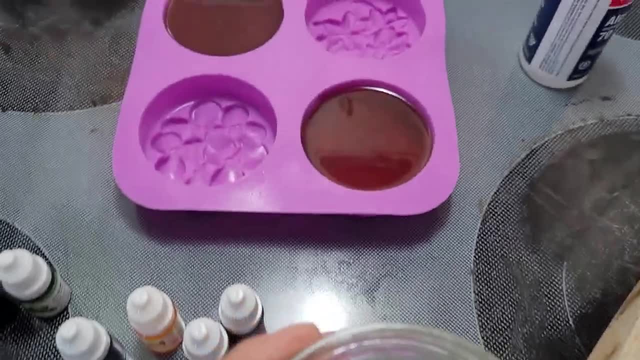 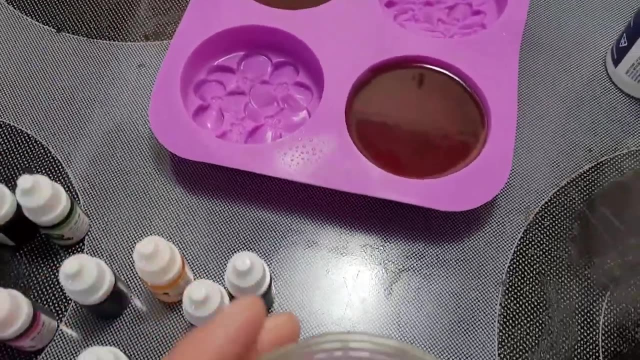 different. I'm going to pour in the clear glycerin base into the mold and I remember to spray the mold bottom with alcohol. this time I'm going to maybe try doing a few little drips of different colors and like swirling them throughout and see how that looks. this is so fun. I love experimenting. 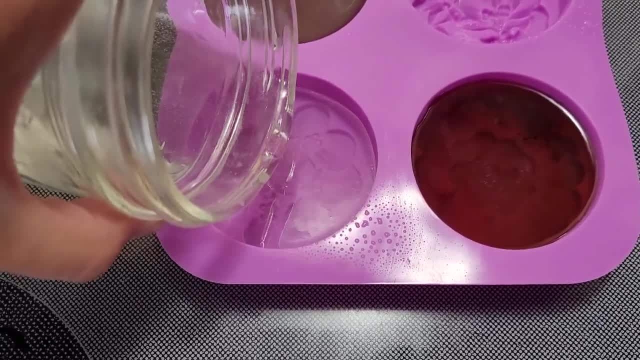 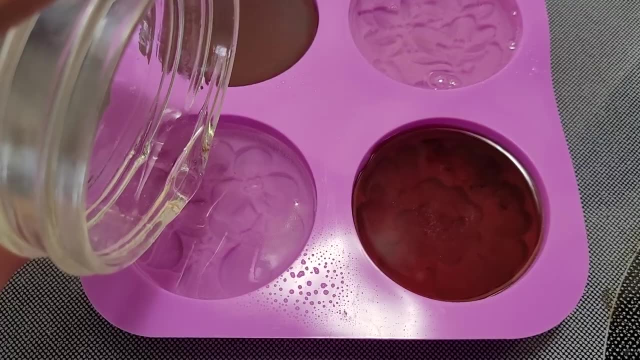 um, you can't do anything wrong, really. if you don't like it, just melt it down and do it again, you know. so I'm going to put that in there, that one in here that takes about three cubes for each one of these. okay, that's pretty good. now let's experiment, all right, so I'm just gonna do a. 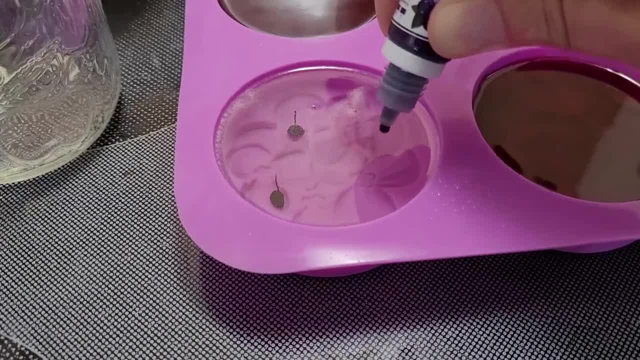 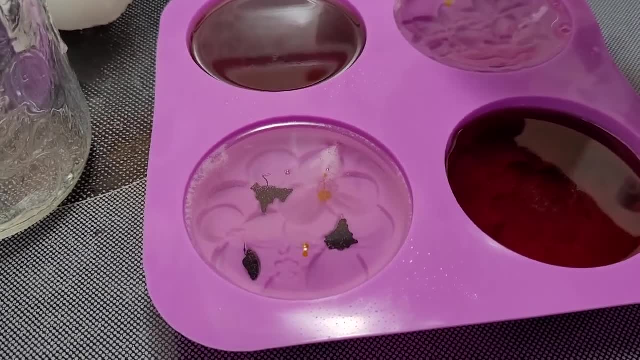 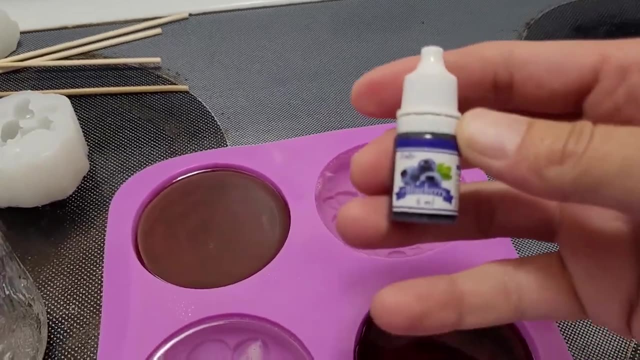 couple little drips so kind of heavier. oh, look at that, that's cool. I'm just gonna do like little swirls. eventually I'll get my little stir stick a little bit of yellows in this one. I don't know what do we got here? oh, we got some blueberry. let's do that one. I work fast before. 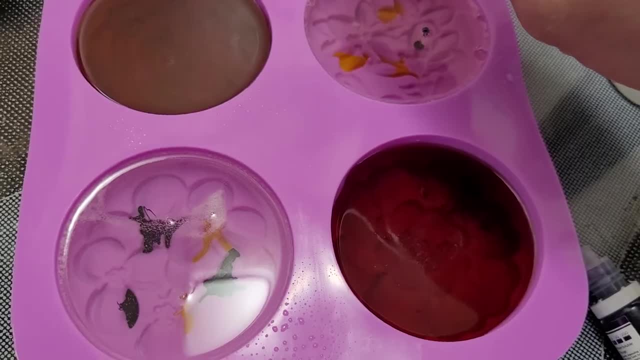 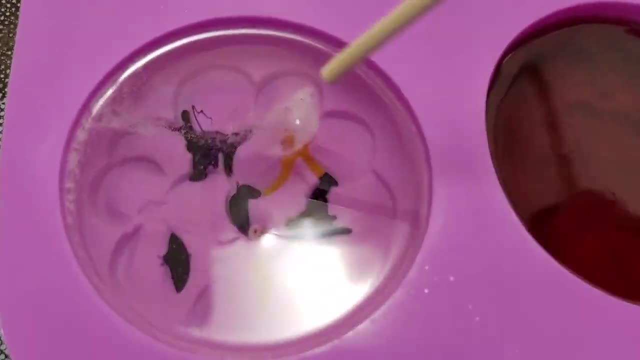 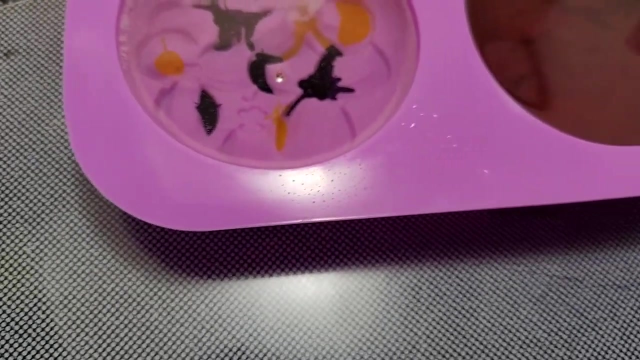 this starts to kind of settle up. all right, I don't know, this might be a bad idea, let's experiment guys. hey look, it's a kind of falling into the um, the flower pattern there. look at, you could probably I'd get some in the actual petal zone there. that's neat. yeah, it's just heavier than. 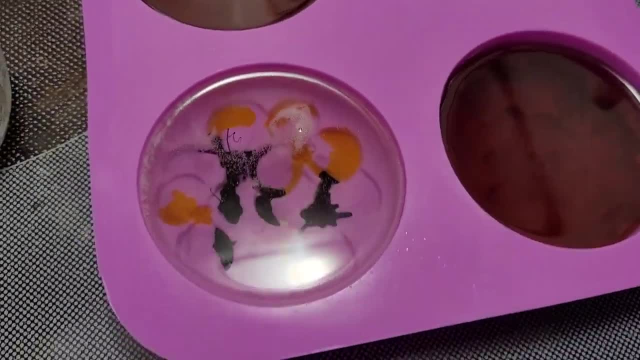 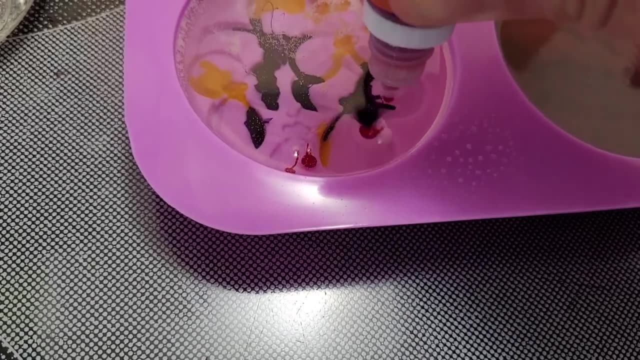 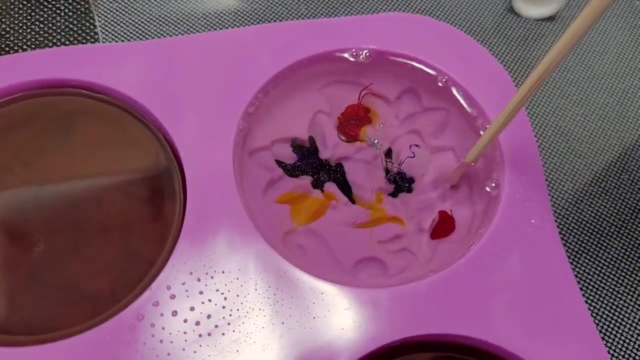 the uh glycerin base there. so isn't that that's cool? I didn't know it did that. that's another way you can kind of experiment with it, see what it looks like. of course, that uses a lot of your dye. I like that. it's kind of cool. so, yeah, this one, I'm going to try to swirling it around see what it. 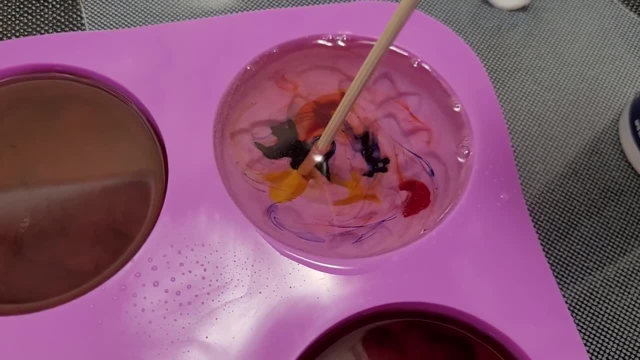 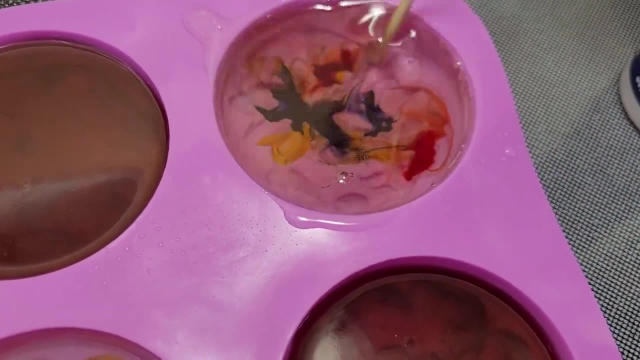 does, maybe letting it set with some of the swirls, like not completely mixing it, a tie dye, look, and it's going to be heavier, so you can see it'll sort of rest at the bottom in the pattern. so I'm kind of just painting with it in here. so that's interesting. 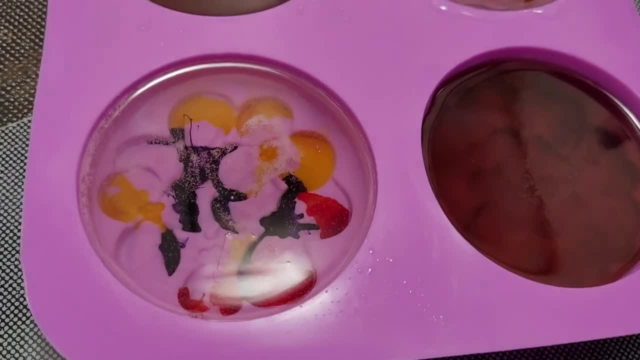 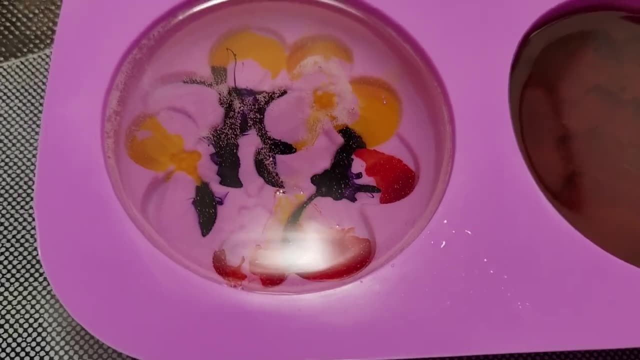 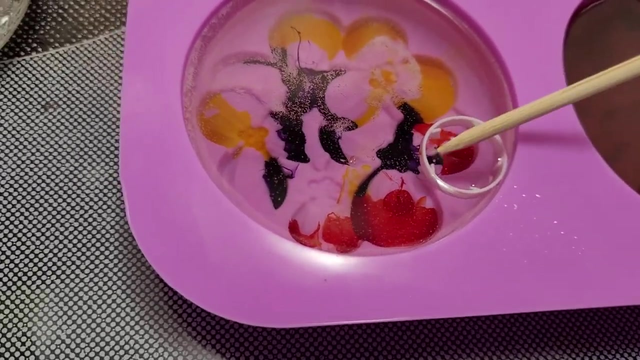 I'm learning something here, and this one I'm actually- you know what I'm actually going to practice like not mixing it up, I'm just going to see what it's going to do if I kind of let it get into the mold there. more of the red there for that. oh geez, that's not good ah. 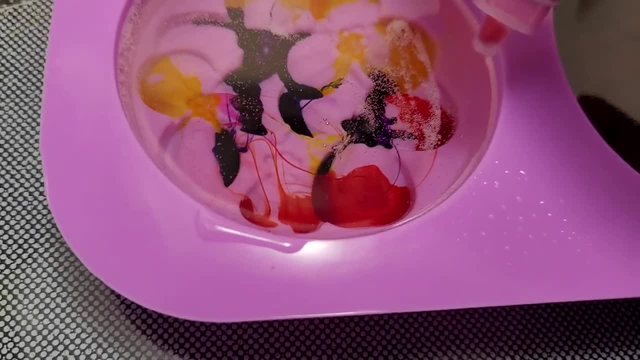 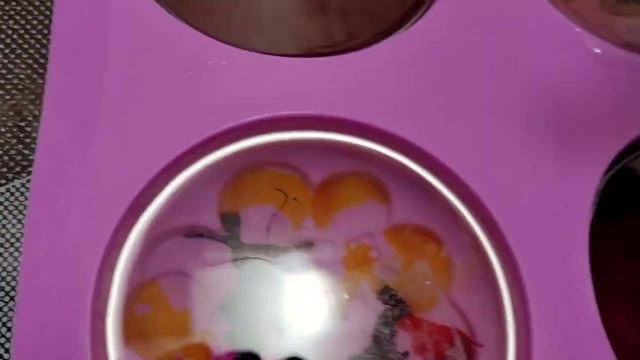 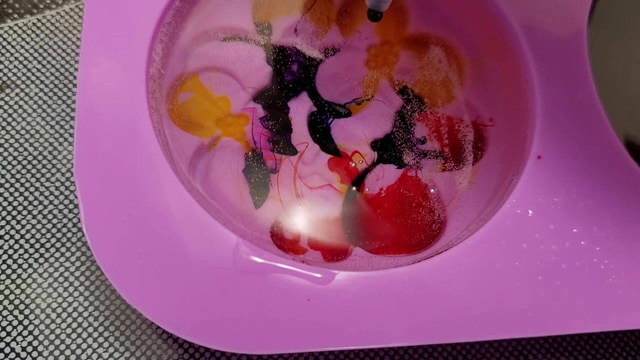 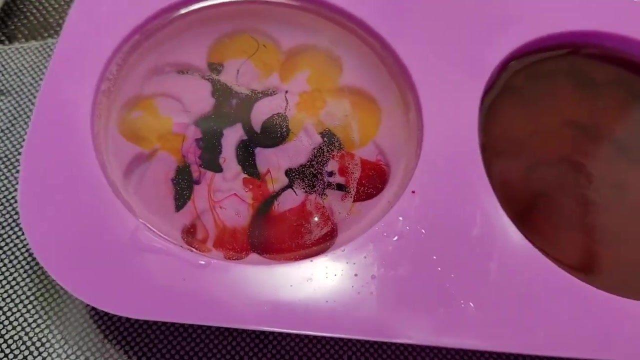 outtake, um, so I'm going to stick it down there, get it into the petal. there we go, take this one a little bit more, kind of like a really pretty pansy or something. well, this is quite the art experiment, let me tell you, okay. and then, when you're kind of 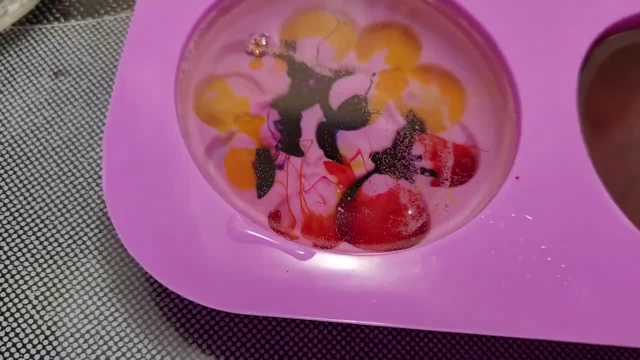 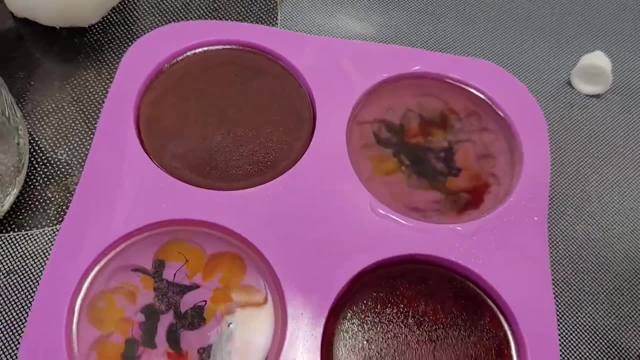 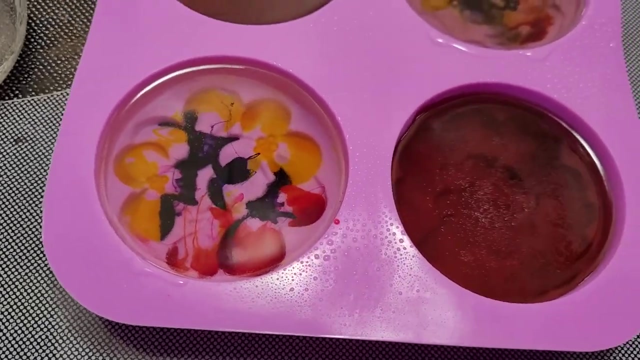 um, happy with what you got. then don't forget to spray it again with uh alcohol. yeah, that one wouldn't be as weird if I hadn't dropped the uh the top in there. okay, so now we're just gonna spray it to burst those little itty bitty bubbles on the surface. break them up. okay, good enough, okay, great. 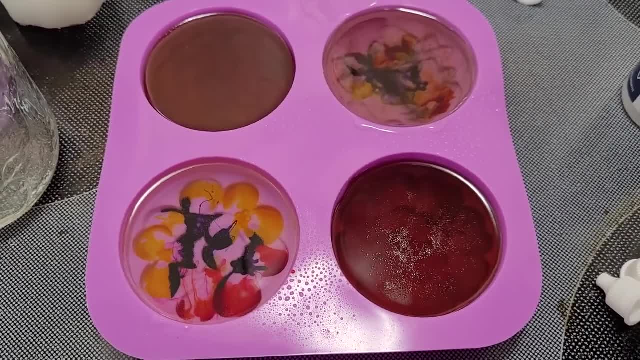 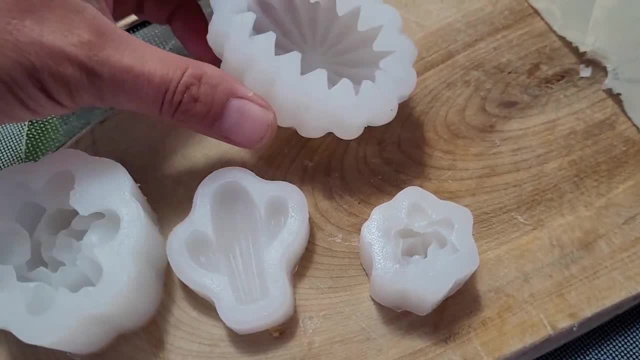 so we're gonna let this set now for a couple hours. let's go on and make the rest of our soaps. next one's going to work with are my little succulent molds. I think these are gonna be really cute. um, you know, if you have like guests over and stuff like that, there's. 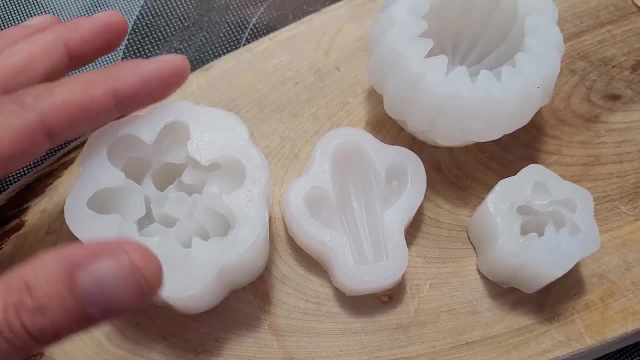 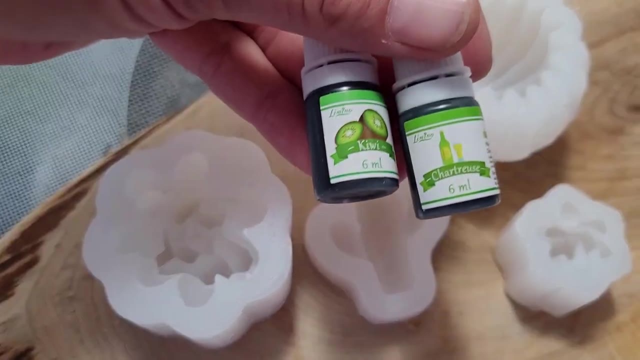 lots of different molds you can get online. um, so I'm gonna die. uh, use these dies here. so I've got chartreuse and kiwi. I mean they look fairly similar to me. um, so we'll kind of make a line for these cactus molds, all right, so I'm not gonna go light on this stuff at all. so again you. 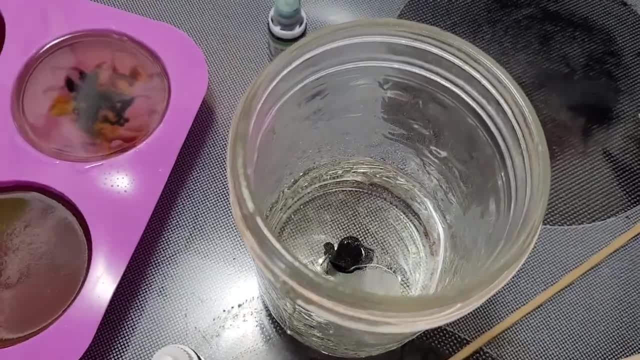 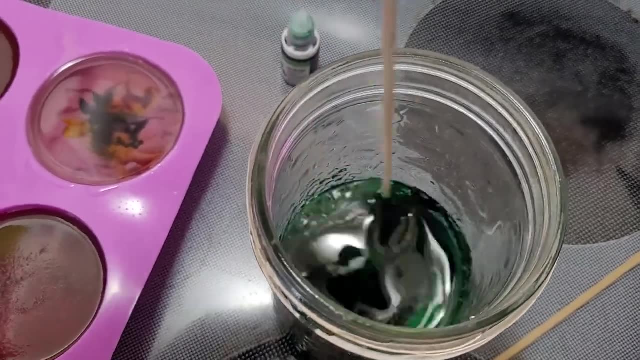 can put in your essential oils at this point, and you can put in your dies again. everything has to be for um, soaps, um, and safe. oh, there's a little bit that's not melted. I'm gonna pop this in the microwave for a couple seconds, but oh, that's the color I want, perfect, all right, two more seconds. 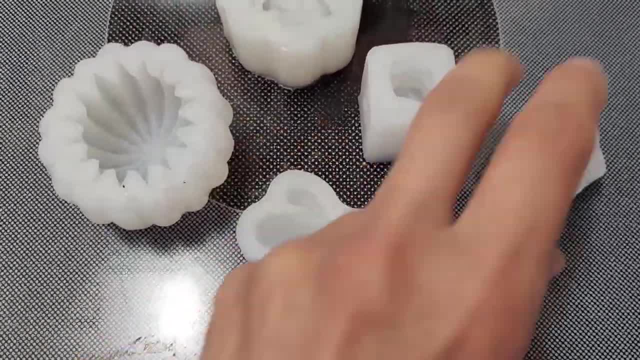 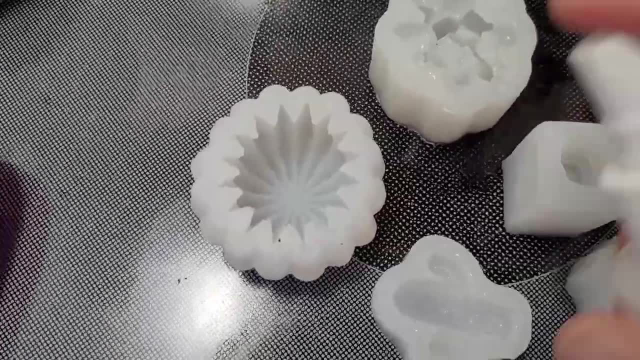 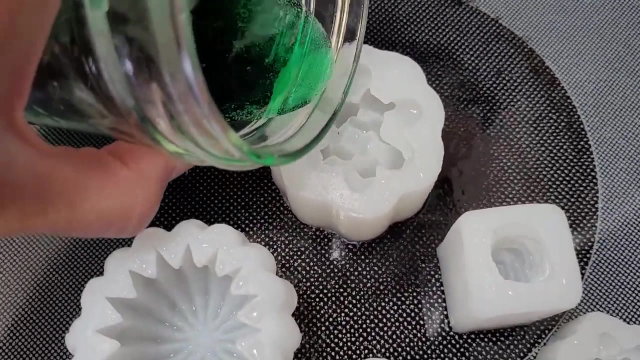 in the microwave and we should be ready to pour. so got these all out here. remember um again sprayed inside of these things with alcohol, because there will be bubbles in this kind of a setup for sure, and then we're just gently going to pour in um mold here. 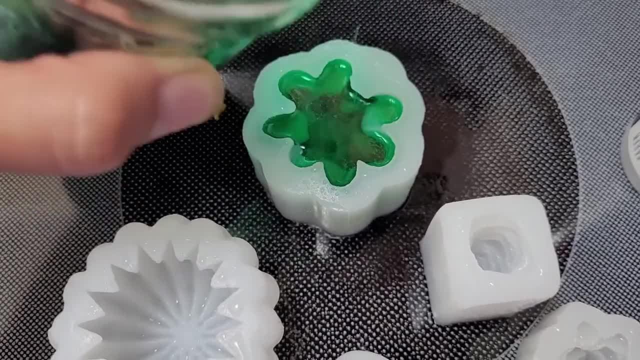 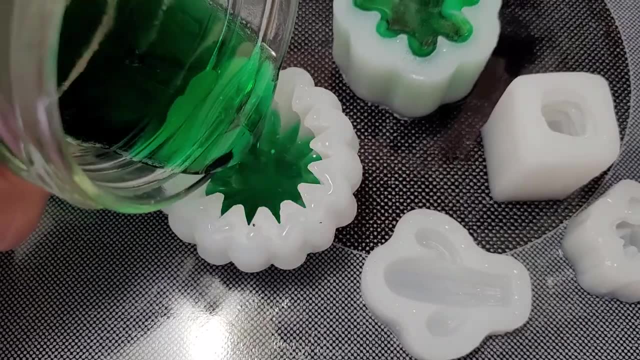 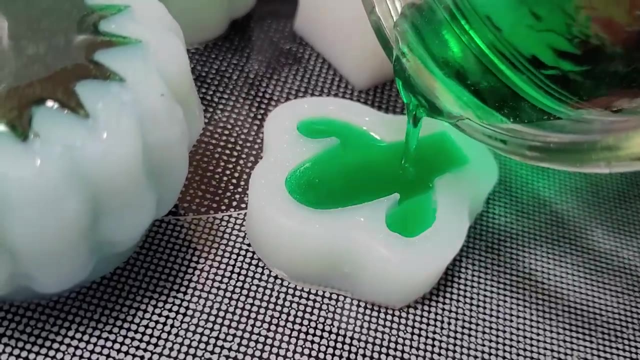 these ones don't hold as much as you'd think, so just be careful, and that one's- this will be obvious- excited, oh, to see how this is going to turn out. again, it's really fun wearing gloves. see that one's really small, and well, those are setting. last but not least, I'm 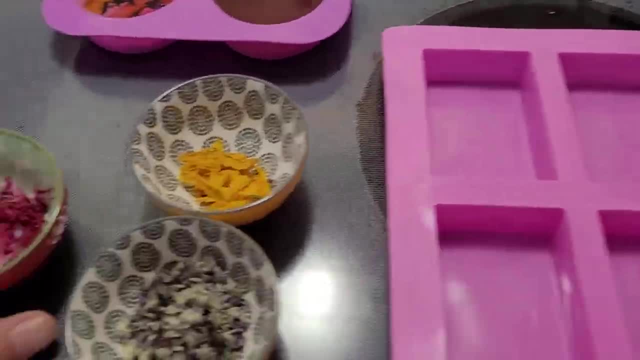 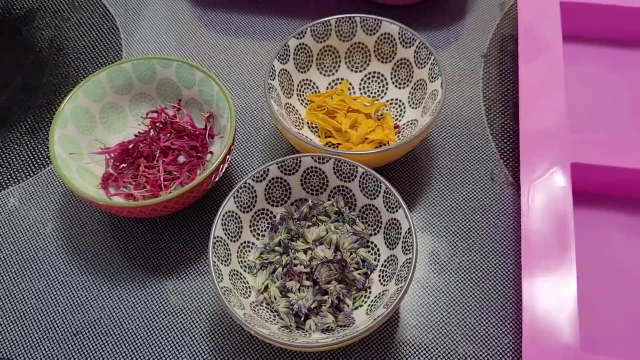 this is the part I'm most excited about. this is doing the clear soaps with my fresh garden dried flower petals. this is really exciting. um, the glycerin I bought is, uh, ultra clear, like 10 out of 10 for clarity. now you can see how clear these bars are, so we're gonna be able to see the flowers. 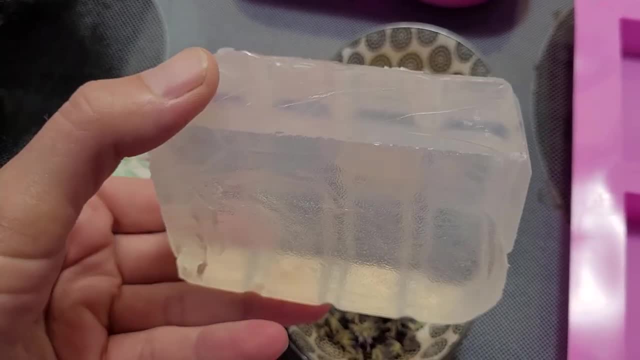 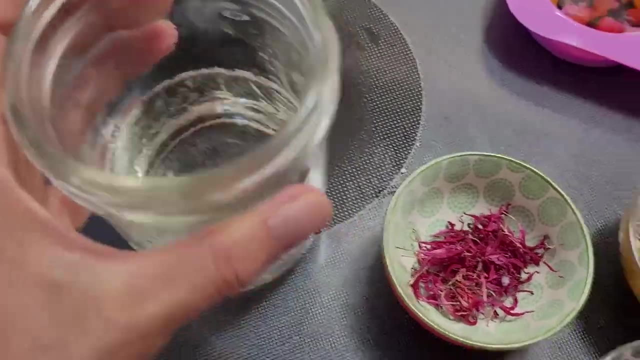 throughout. so this is really awesome, important. uh, use dry flower petals and it works so much better and doesn't get all yucky. so I've melted- um, you know, some more right here. let's work in little batches. so what I want to do is just I'm. 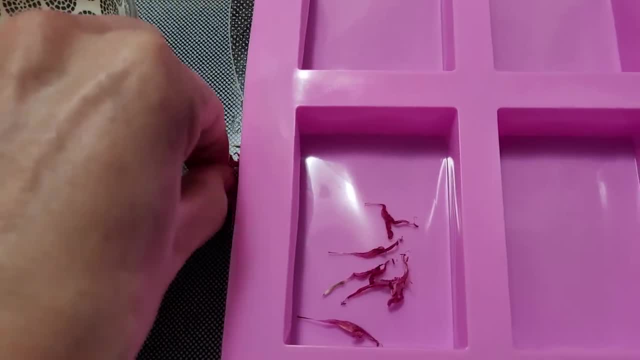 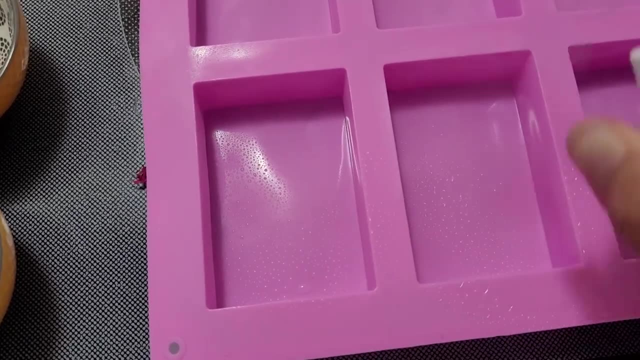 going to start and maybe pouring this in layers. just do a little bit here. oh geez, alcohol spray. I always forget. all right, so we're gonna start by doing a little bit of alcohol spray again in our mold for the bubbles. and I'm just going to start, maybe just in a few little layers, we're just going. 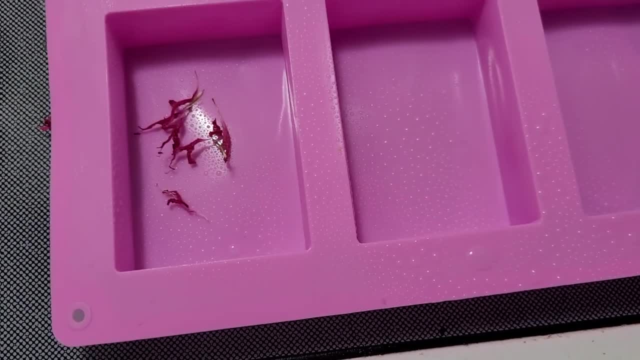 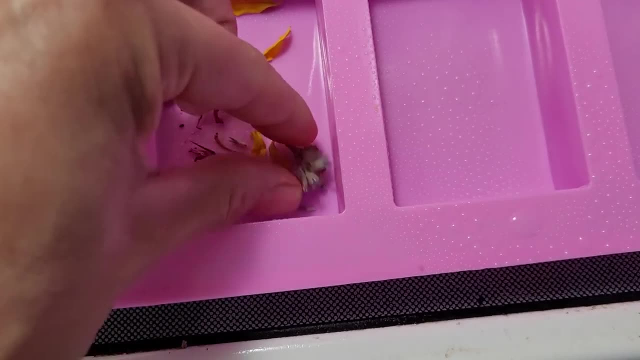 to do a little bit here and you can be as creative as you want. this is what I love about this: you can be a unique individual. these are great Christmas presents, bridal shower presents. if you have kids, you might want to get like those little plastic toys or something and stick one in the middle. 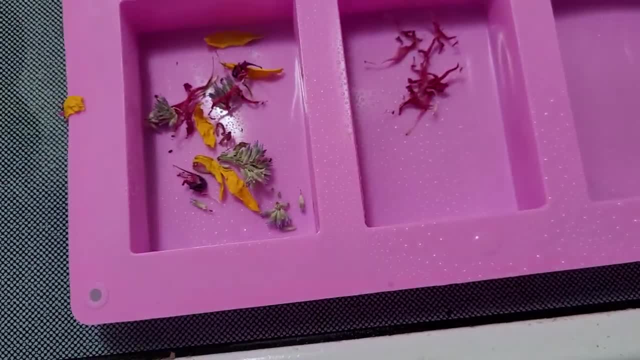 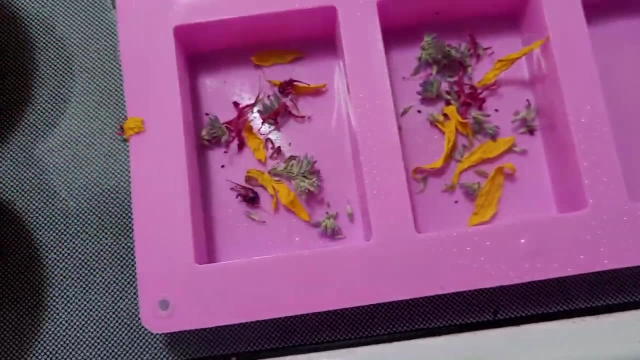 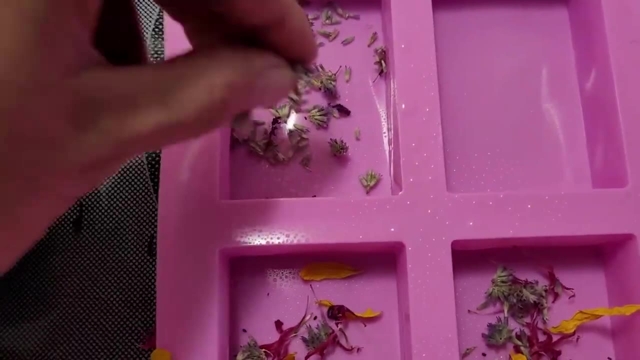 as it's partially setting. that'd be kind of cool. um, so, like you can do so many cool things with this, there you go. I mean this one, I mean I might just do one straight with a knee- so you want to use, like you know, an essential oil, um, like kind of like licorice, or smells licorice. that would be the one to use for. 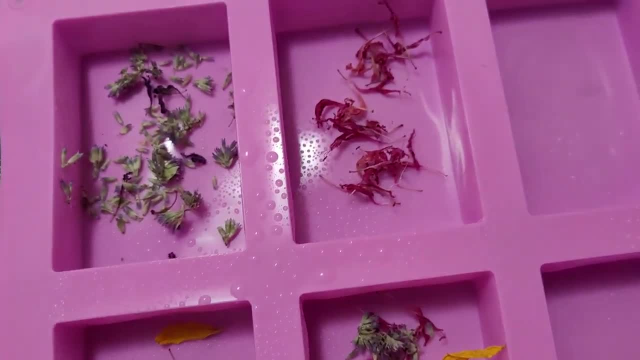 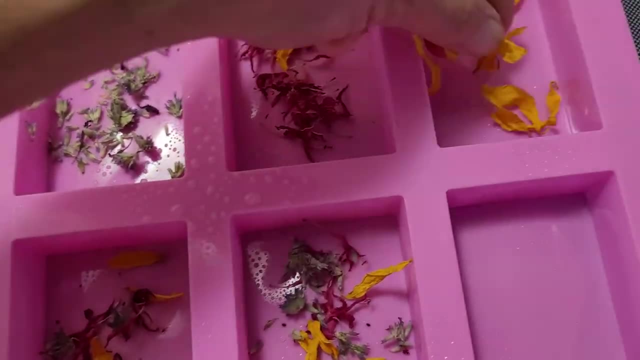 bee balm. I'll say this one right here. it smells mostly like oregano, so they're. that's another idea. again, I'm really scent sensitive, so I'm just leaving these plain, just gonna kind of fill all these up here. I don't know if they'll do all in this first pour, but 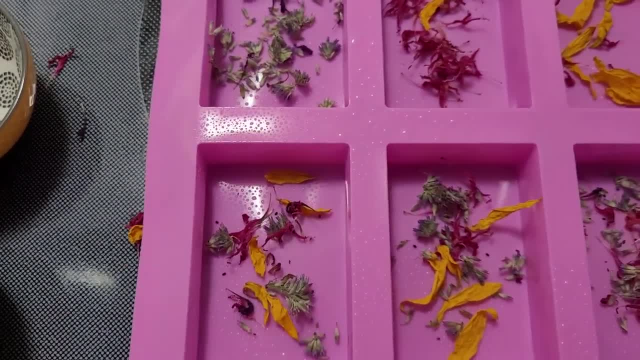 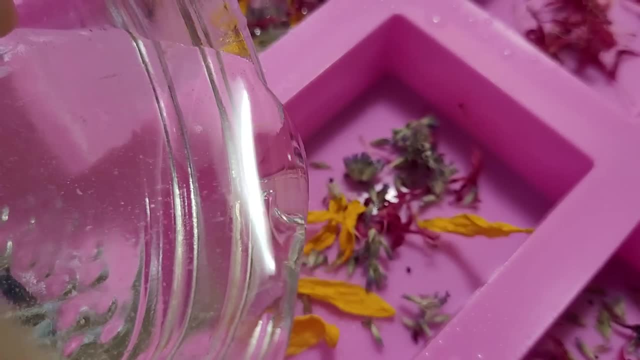 all right, that's a good bit to get started with. let's uh, let's start this, see how it goes. it's always going to move around, and that's why I've got my little um stir stick to kind of uh, push this around after. so don't arrange it until. 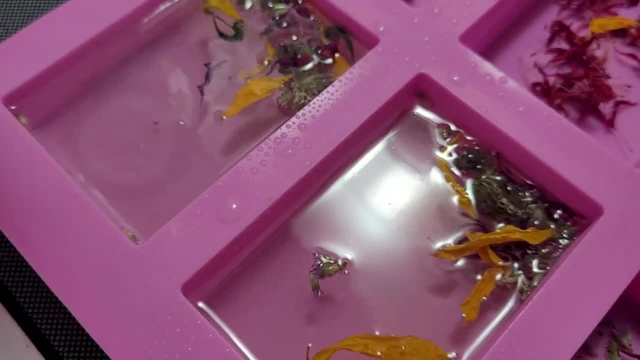 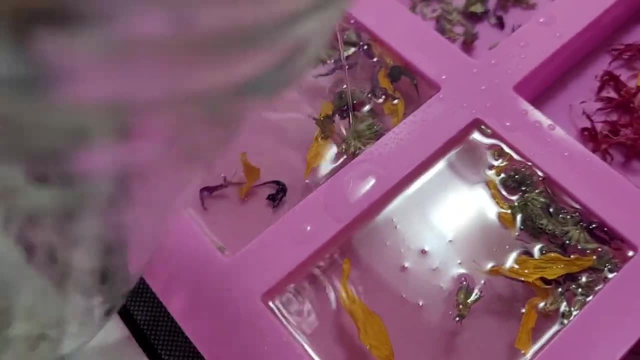 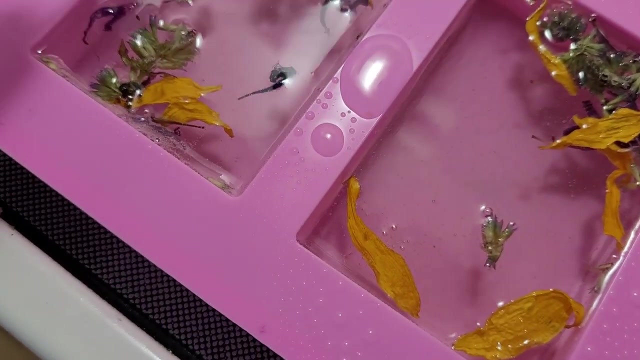 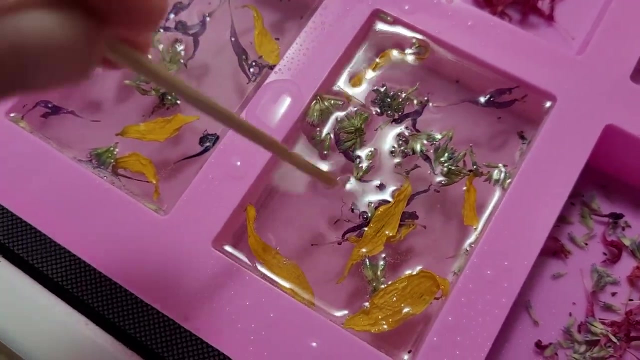 after the fact, I can get two bars out of this, so I got a smaller mold too, all right, so let's push this around with my little stick here. so these are probably going to want to floats when I'm learning here. so that's okay, just move them around, just to how you want them to be. still, look super pretty. look at that. 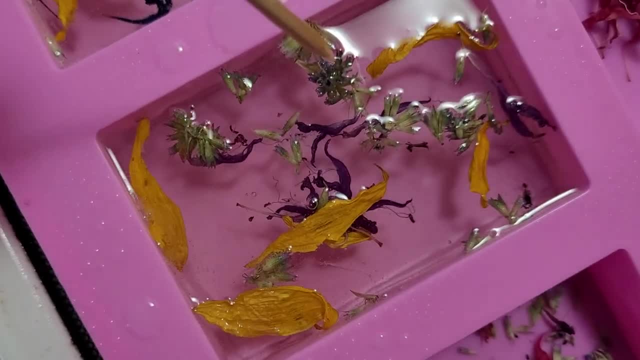 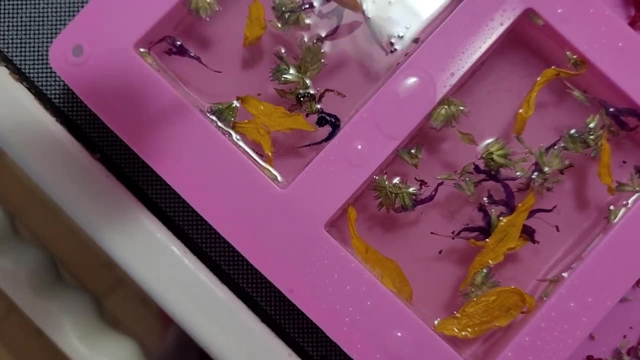 hard to see with the glare on there. but there you go, very, very pretty this thing set. you can kind of maybe push them down a little bit more as it gets a little bit thicker, so maybe we'll do that in a minute. let me get a bit more soap base. looks like I may be able to do. 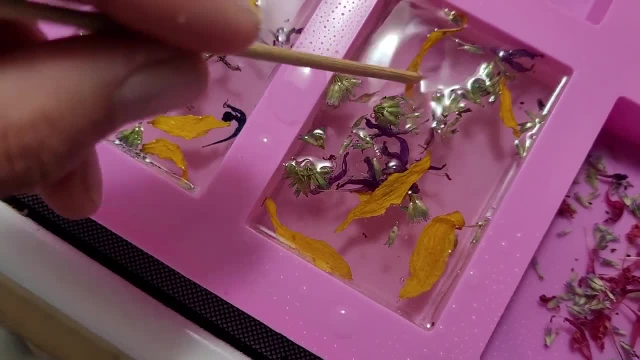 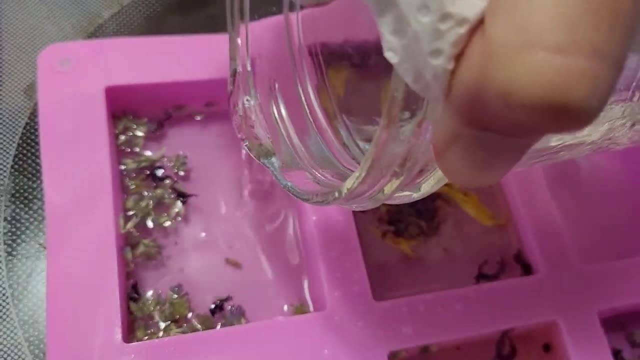 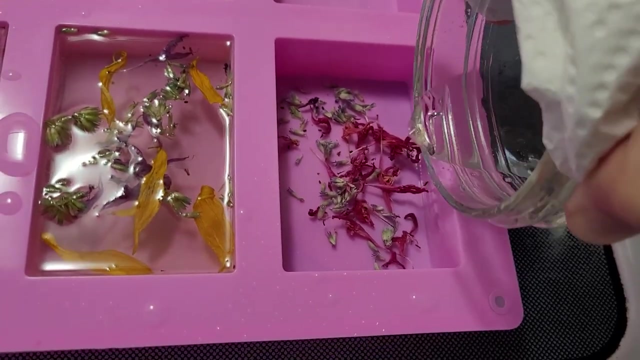 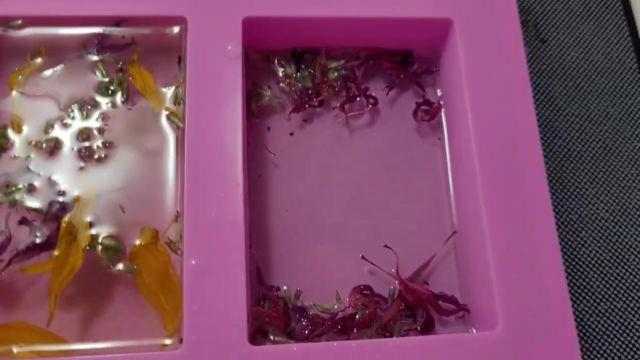 maybe two more with what I bought. I bought two pounds of the soap base, so all right, this might only get a really small little borrowed of, so let's just put whatever we have left over in there, and that's okay too. now some of the star nice has some seeds in. 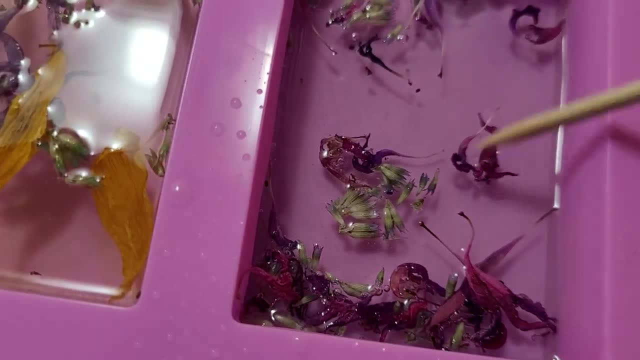 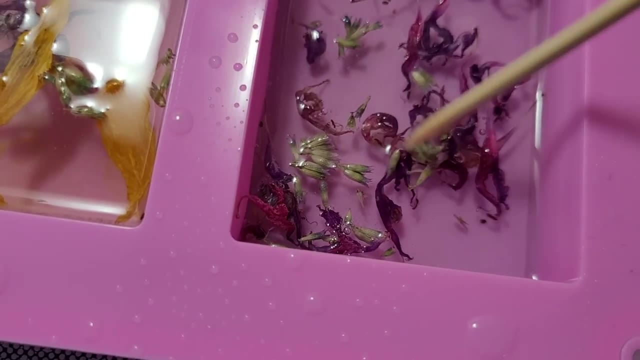 it. so you'll see some little black flecks. that's just seeds, actually, so that's really cool, all right. so this one, like I said, it's gonna be like a half bar, and that's all right. we'll just kind of move this around, make it all pretty and this one is purely star anise. 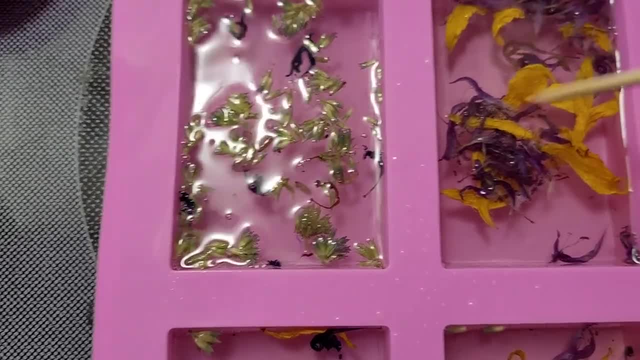 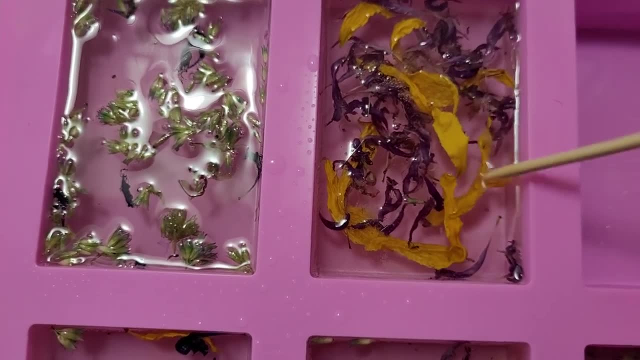 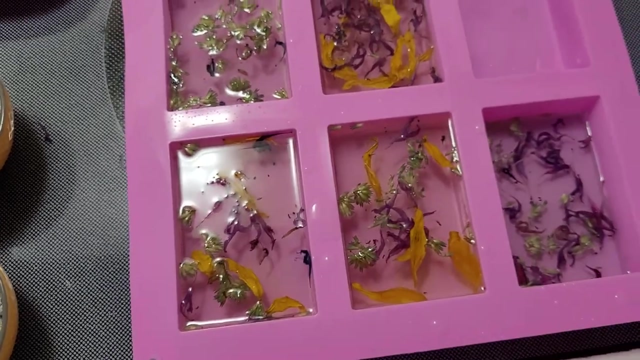 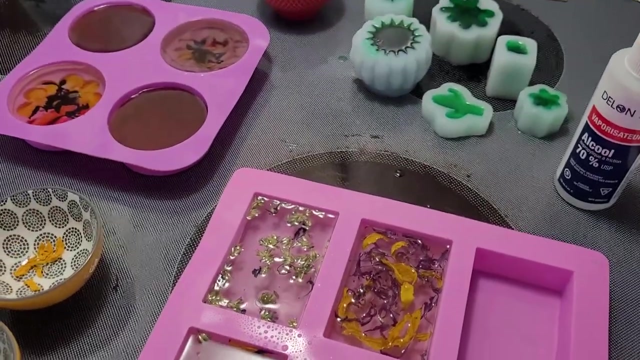 this one has black eyed susan and the bee balm. oh, that's cool like that. very good, all right. so when you're happy with your arrangement, make sure again. just do little spritz with rubbing alcohol so don't get the bubbles. now we're gonna let all of our soap sit for a couple. 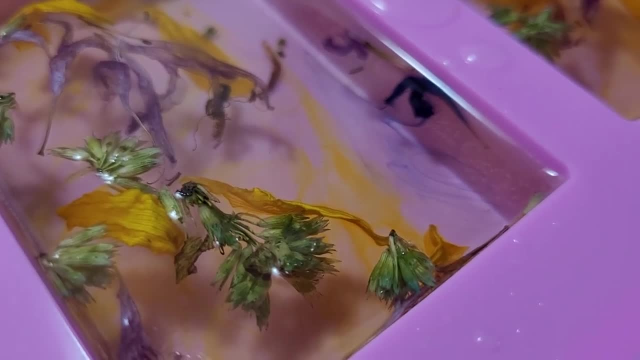 hours and we'll check back in with you. they've been setting for about maybe 15 minutes or so and then we're going to let it sit for a couple hours and we'll check back in with you. they've been setting for about maybe 15. 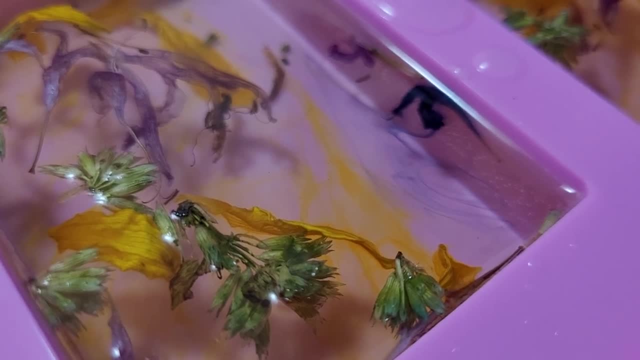 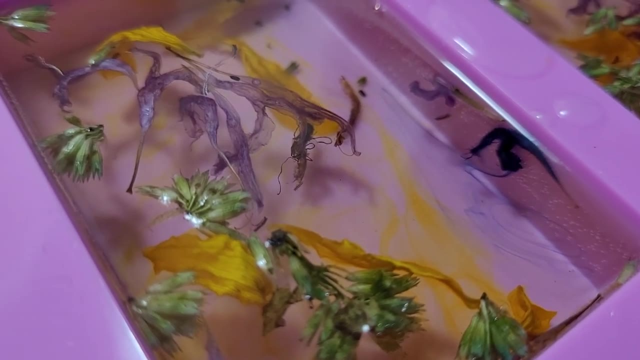 20 minutes. I want to show you a really cool thing that's been happening, as you can see there, with the bee balm in that little purple bit there. it's really interesting. the bee balm has turned purple in this glycerin soap base, which. 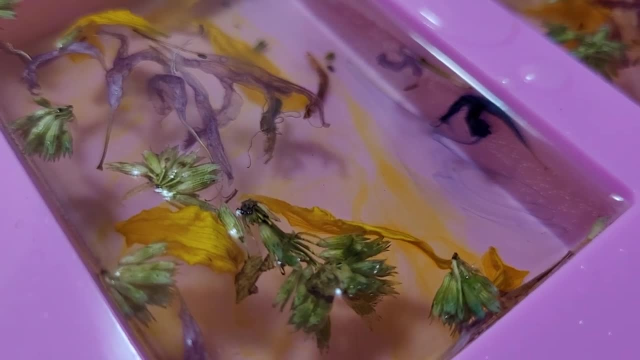 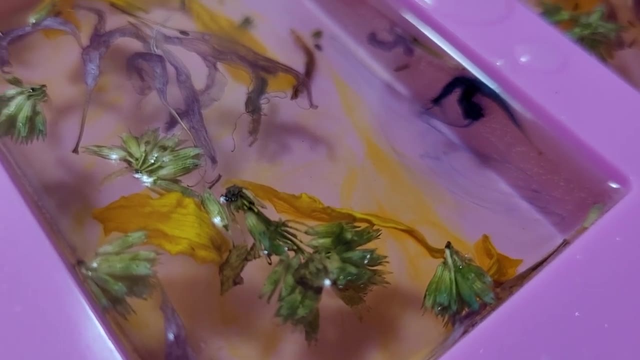 tells me. you know it's an acid base indicator, so that's really cool. so it's changed color. it's not the pink that it used to be and it's giving off a purple dye and, as well as the black eyed susan petals, it's giving off a yellow dye. so 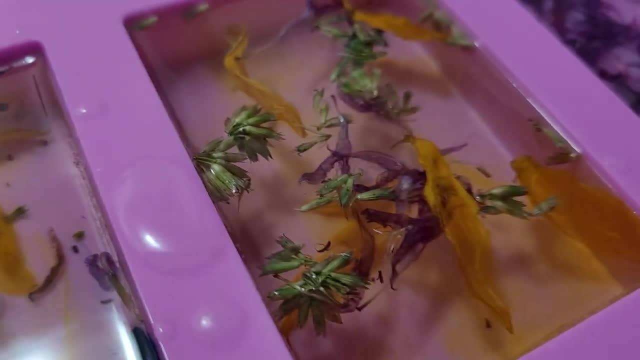 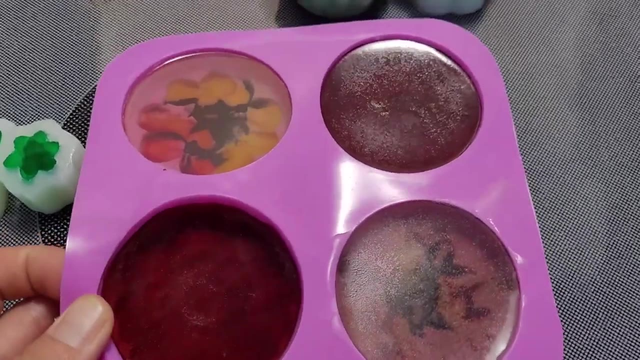 very natural dyes for the soap, so that's something to consider as well. if you want to make some natural color changes to these soap bars, the flowers will do it for you, okay. so we're about an hour and a half, two hours later. let's do the big reveal. so I'm gonna 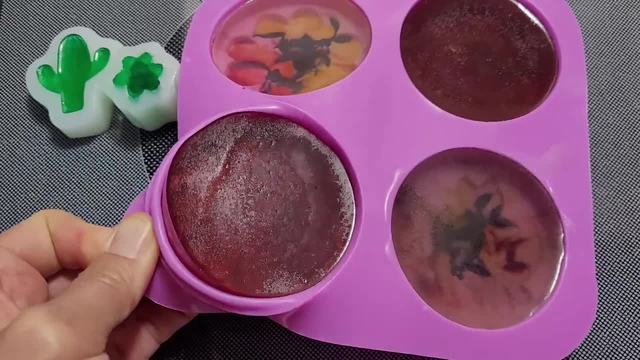 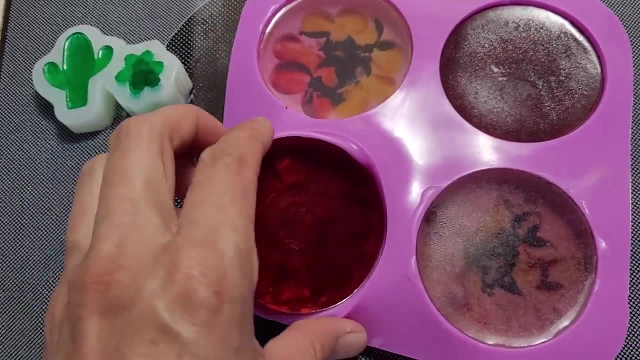 start with these ones right here. so it's pretty easy: just peel them out of the silicone mold like this, and they really just kind of like pop out. so we're gonna take a look. this is the one I did the red dye in to kind of make it look like. 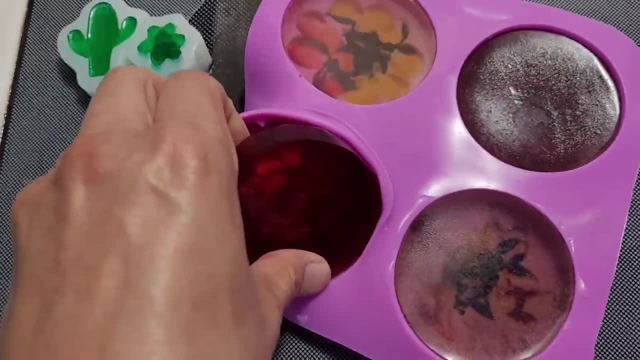 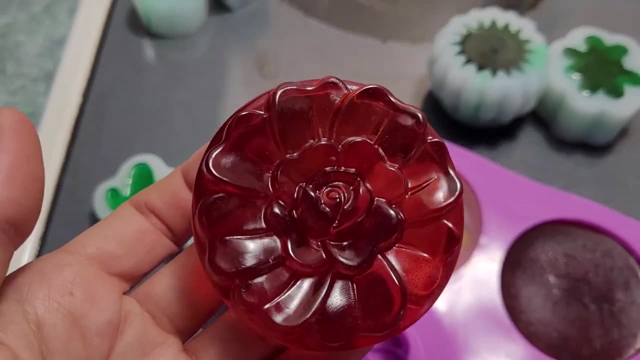 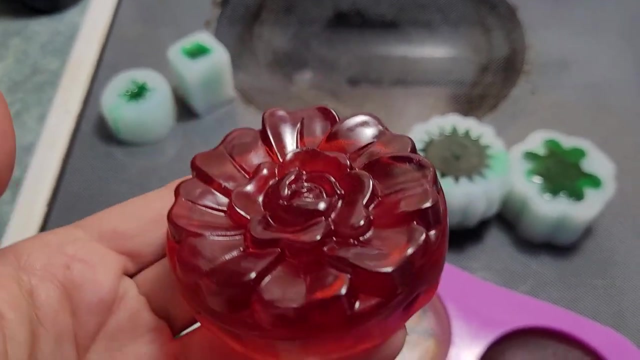 a rose. let's see here: whoa, that's beautiful. look at that, absolutely gorgeous. the clarity is amazing, like look at that through the light. so that's beautiful. let's take a look. the rest alright. so I took this one out with the food coloring and this one didn't turn out as expected, I think I 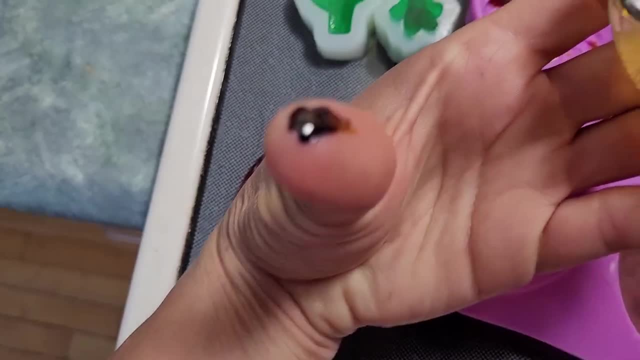 really should have premixed that. so there's a bit of food coloring kind of stuck at the top. so don't do as I do with that, mix it throughout. but I think some of it did in here and it's really pretty. just some of this purple didn't. 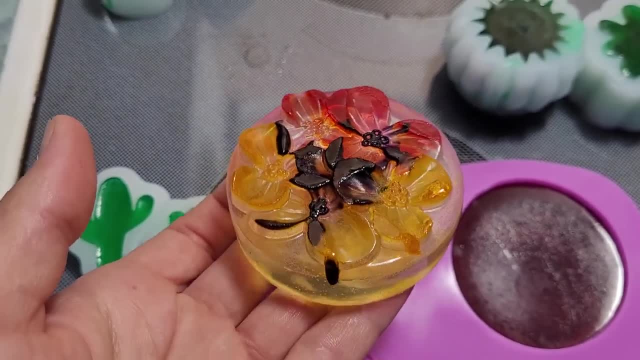 so that'll rinse off really well. again, it's just soap, it's just gonna wash off. you may want to keep that one in there a little bit longer and then we'll see if you like the color for yourself and kind of rinse off some of the color again once it's really mixed through it's. 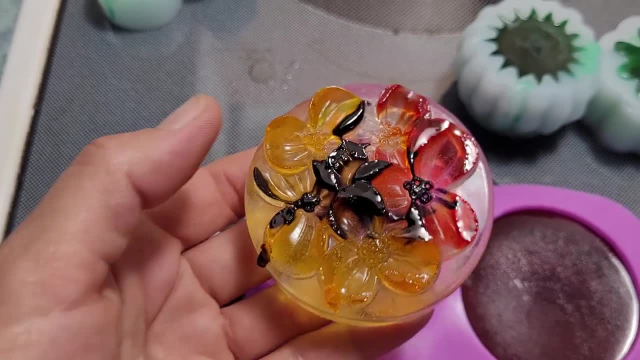 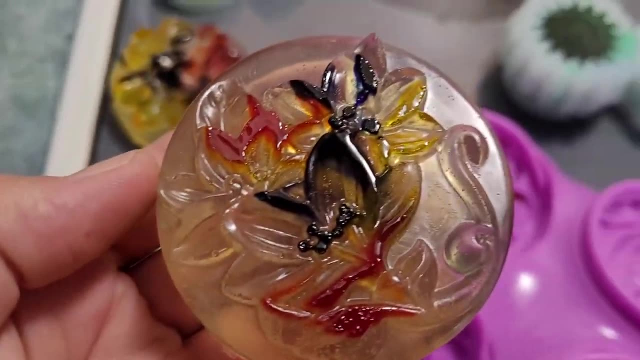 not going to stain or anything. it's just because this has a big glob of it that didn't mix into the glycerin soap base. that's why there's a little bit of stain on my hand. all right. so the other red one turned out really well. on this one not too too bad, but again i don't think i'll do that again. 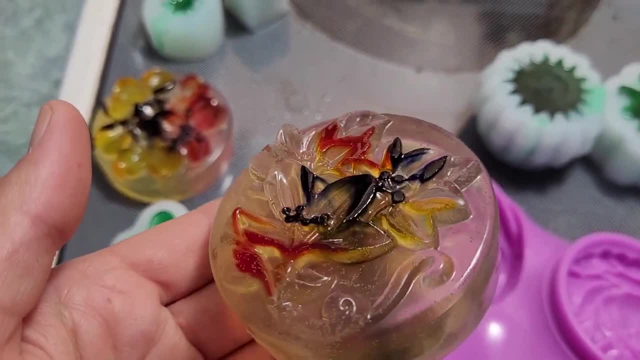 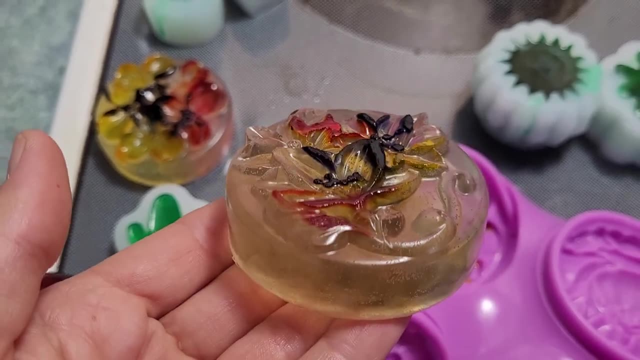 sort of dripping the the color into it. i'll mix it beforehand again. some of it mixed in, but some of it did not, so there's a little bit on the surface there again. if you didn't really like this and you don't want to use this at all, just melt it back down in the microwave. the colors: 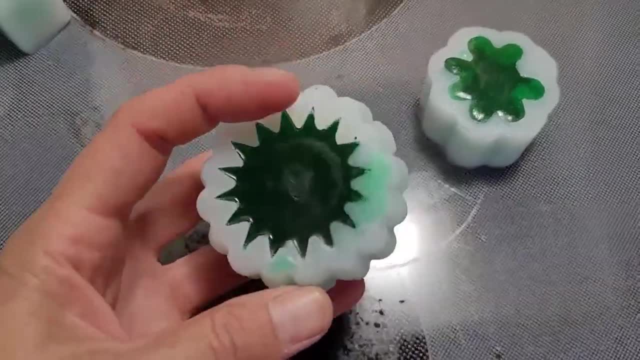 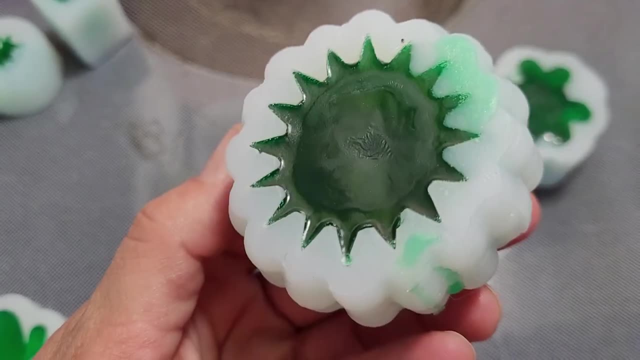 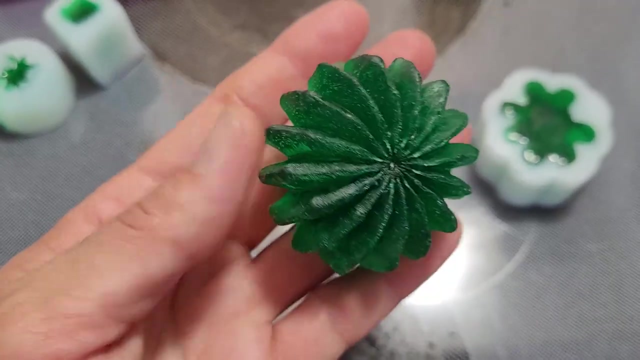 will intermingle and you can re-pour. i am really, really excited, um, for the cactus ones, because you really don't know what you're going to get. this is what i can see, but i don't know what i'm going to find, so let's find out. oh wow, this one's cool. look whoa. look at that. look at the detail on it. 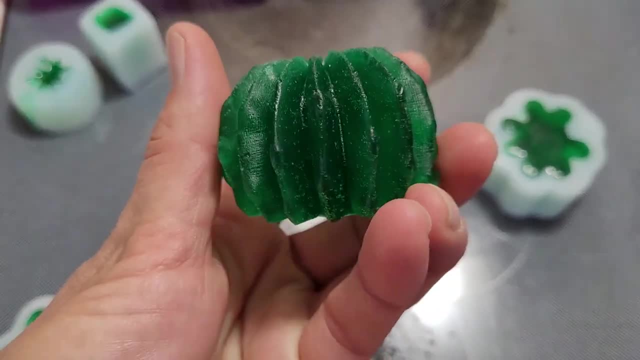 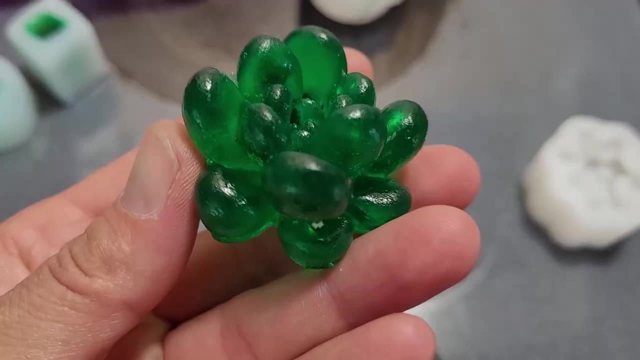 oh, i like that. this is more of your like little decorative soaps you can set up in your bathroom. you can decide whether you want to use it or not. you can decide whether you want to use it or not, give them away as wedding party favors or things like that. so that's one that is really cool. 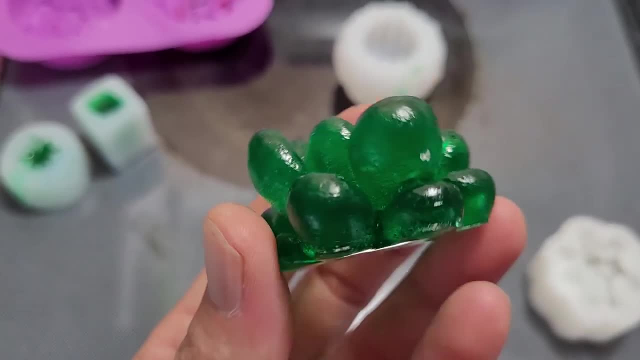 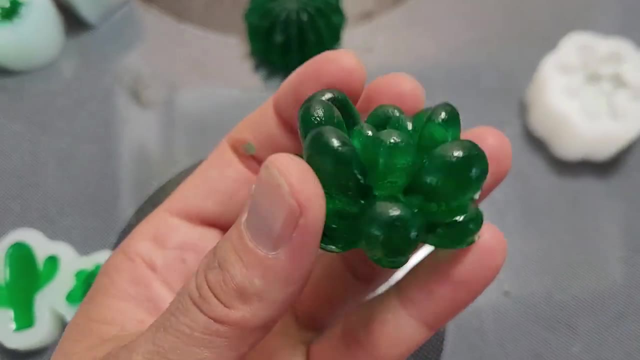 that is amazing. this is perfect for decorative purposes in the bathroom, but it is really functional. always thinks it's something to eat. sad to say, it's not. um, yeah, so, or you know, when you're done with it, you can have these little decorations, melt them down and put them into. 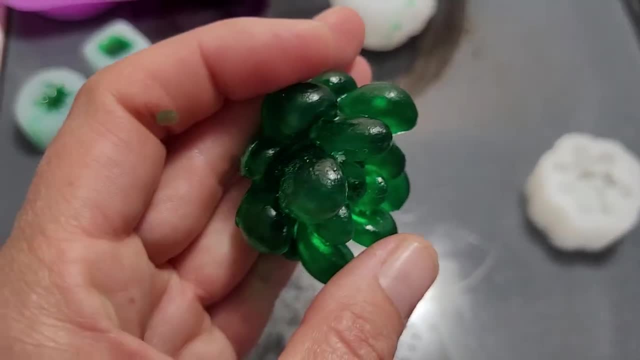 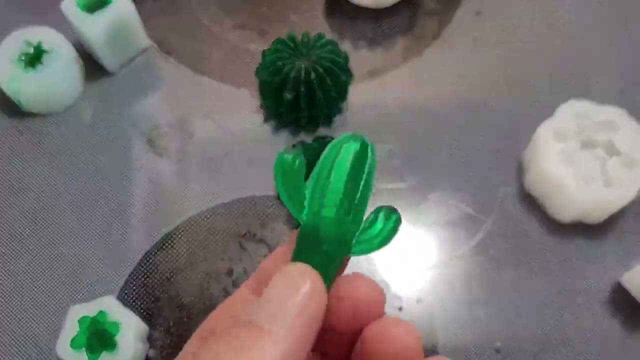 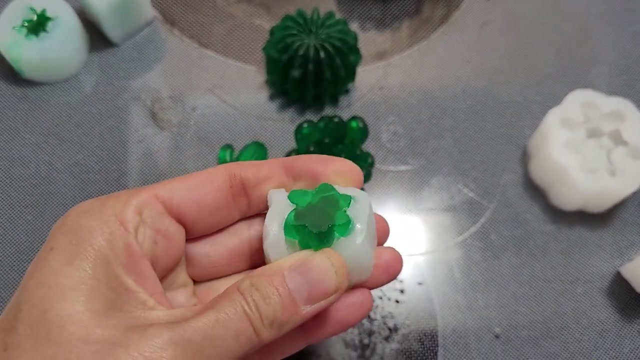 soap that you want to use. i mean, you can certainly use this as soap. it's just got a lot of little knobs on it there. this one- i can tell how that's going to look. that's just a very cute little cactus. i should say these molds can also be used for making candles, so i might do that after this. they have. 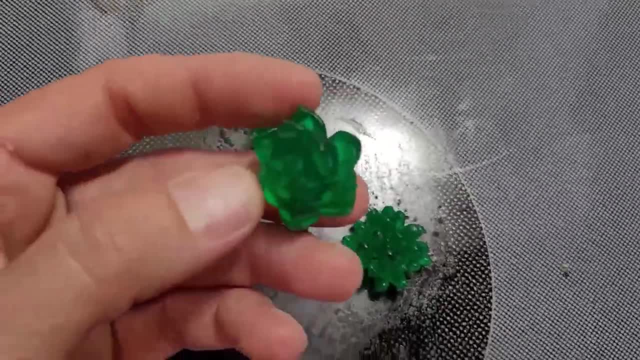 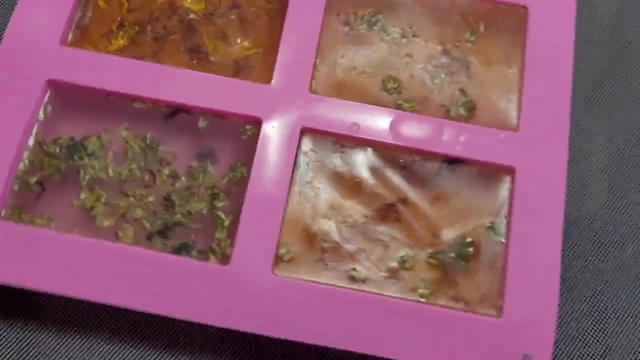 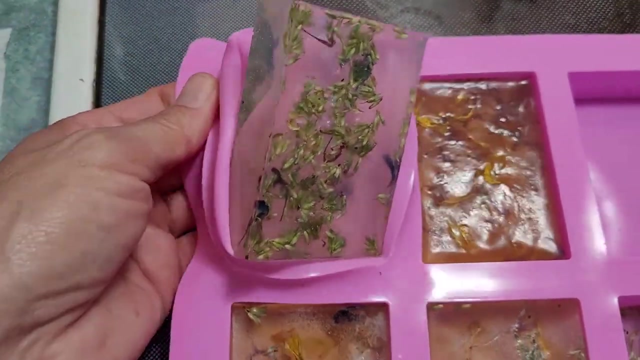 multiple different uses to them. so there's last them. i think they're super cute really: tiny little succulent uh plants there and cacti, so very neat. okay, i'm really looking forward to these ones, as you guys know, um, so let's take a look. these ones are just going to pop out very easily. 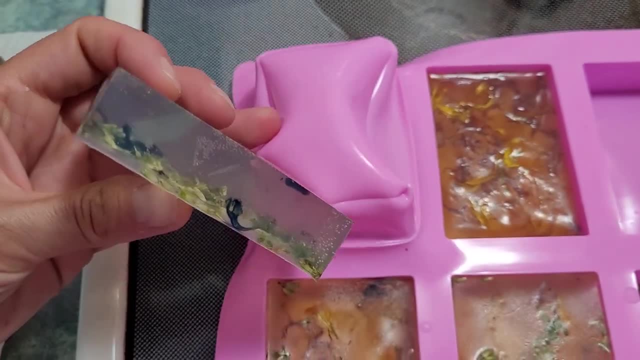 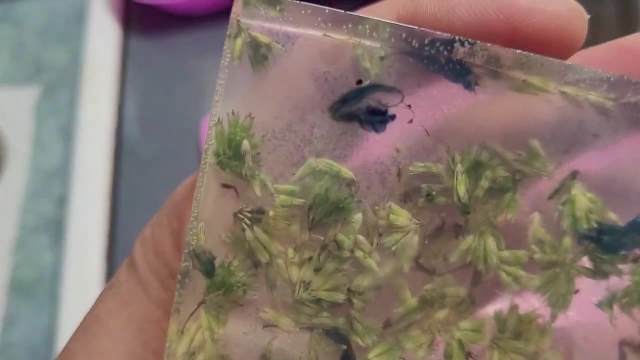 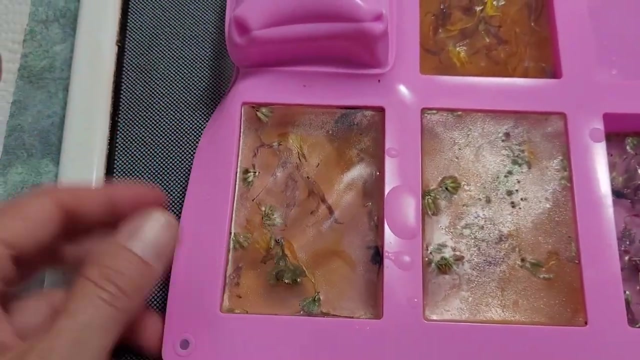 oh, look at the clarity on that. it's like glass almost. oh wow, that's perfect. oh neato, and one of them sunk to the bottoms was actually all the way through great. let's take a look at this one. this one accidentally bumped, so there's a little bit of a ripple in it. that's my fault. i kind of 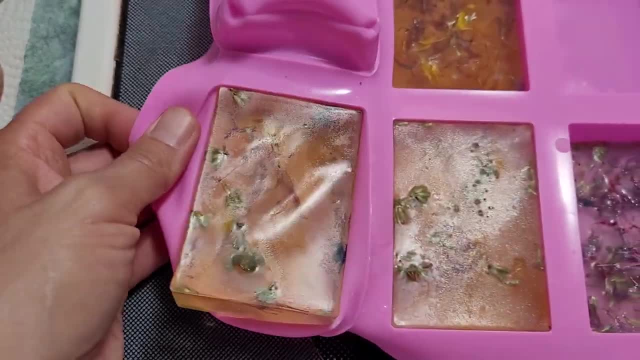 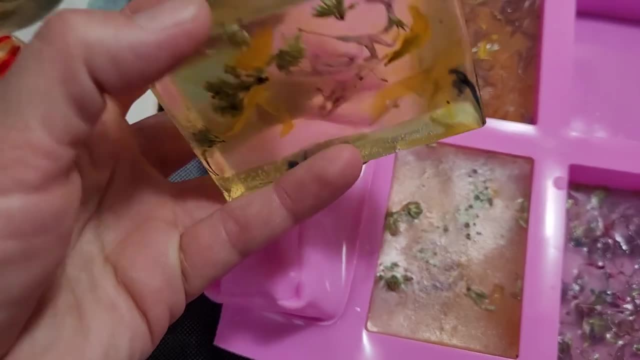 bumped it when it wasn't fully cured yet. so i mean not a big deal soap. so let's take a look. so this has actually got a nice uh yellow hue to it and that is all, uh, because of the uh black eyed hues in there. oh, this is great. look at that. look how clear that is. you can see my hand right. 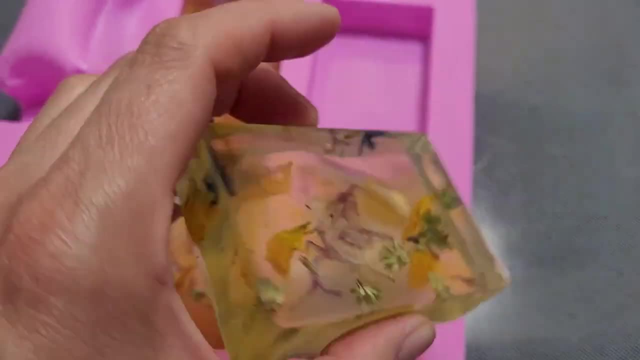 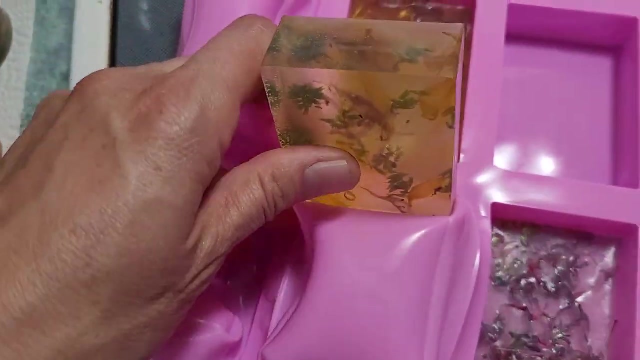 through it and you can see the beautiful flowers. i'll take these outside in a minute so you can truly appreciate it. and again, purples and the yellows mix through on this one, for this is like naturally dyed. i did not stick any colorant in here, so that's natural plant dye in there. and 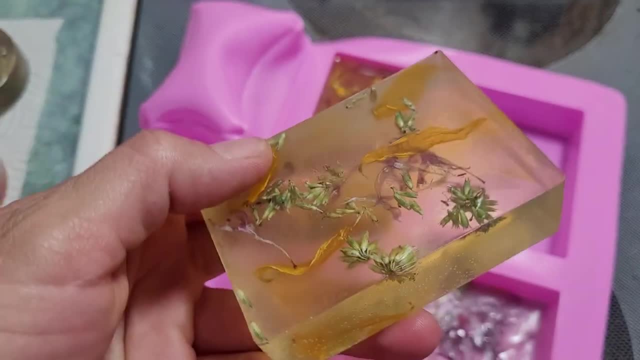 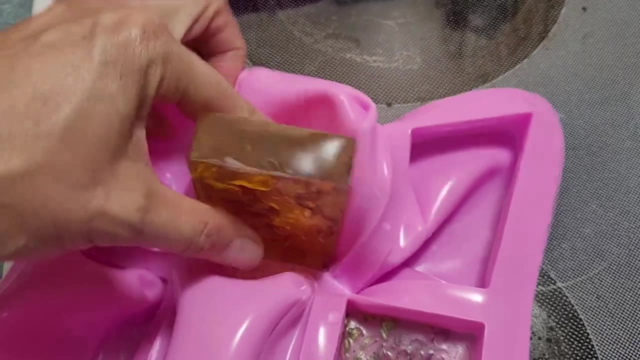 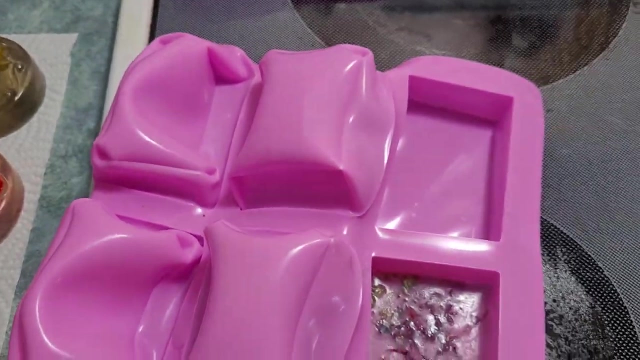 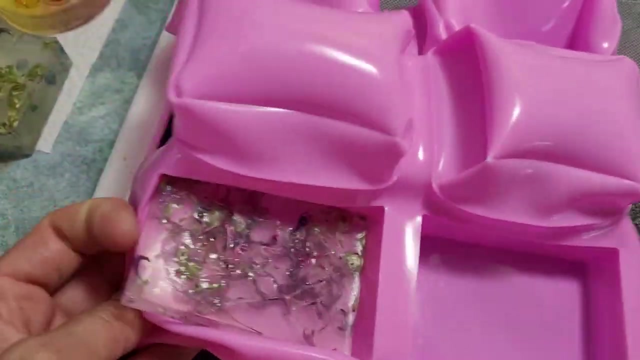 all these plants are. they're not harmful for your skin, don't anything in there that's harmful, just purely decorative. so here we go. there's this one. oh wow, cool. now this one's my little, half-sized one, but that's okay. you know what i actually like it. good for travel. you can kind of cut these. 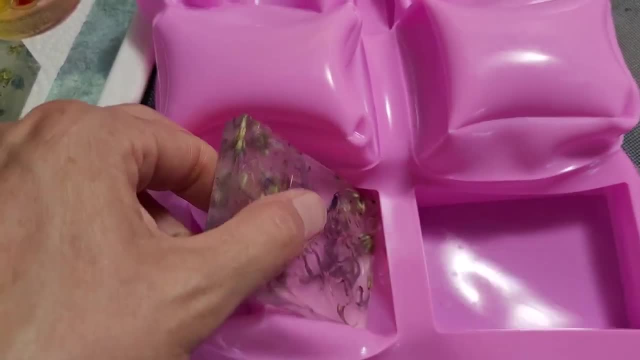 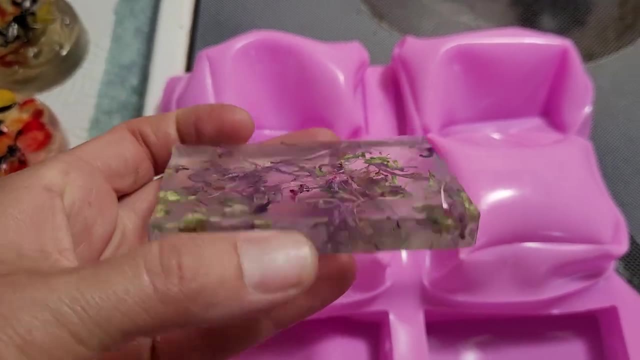 up into little, little, tinier squares, um, to take backpacking or whatever you know, it's all good, just don't wash your hands near a waterway, obviously. but yeah, look at that, isn't that beautiful. okay, let's go outside and take a look at them in the sunlight, these ones.